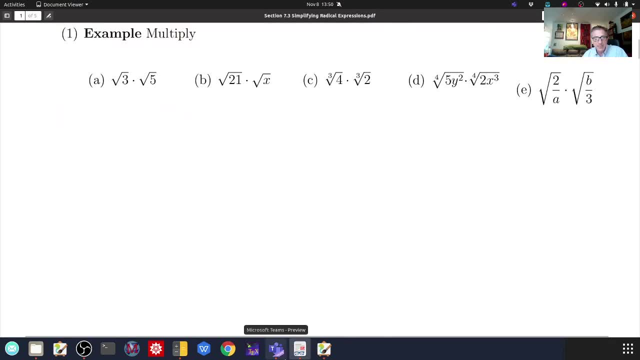 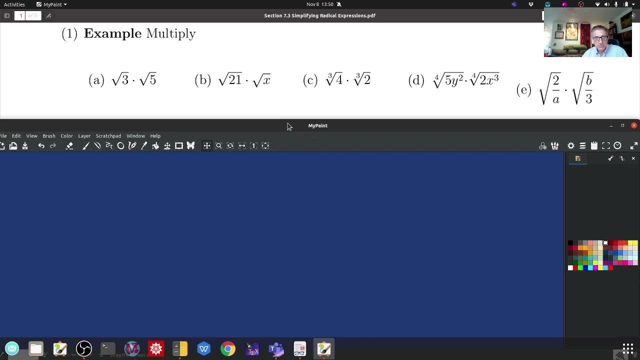 for n has to be the same. So let's do a few exercises. So remember: when no radical is written, it's assumed to be 2.. So the square root of 3 times the square root of 5 could be- if we really wanted to write it that way- is a radical. 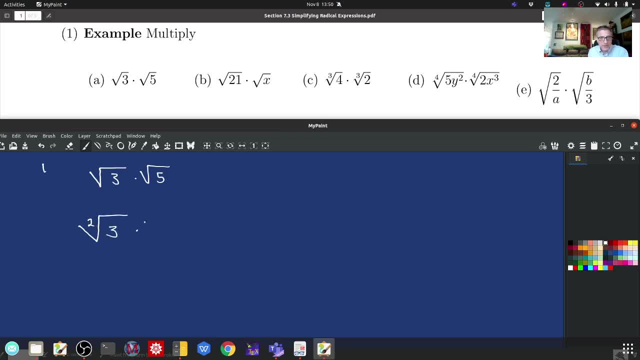 So our index is 2.. The number under the radical is 3.. Our index is 2.. The number under the radical is 4.. So by the product rule for radicals, this is just the square root of 3 times 5. And that's equal to the square root of 15.. 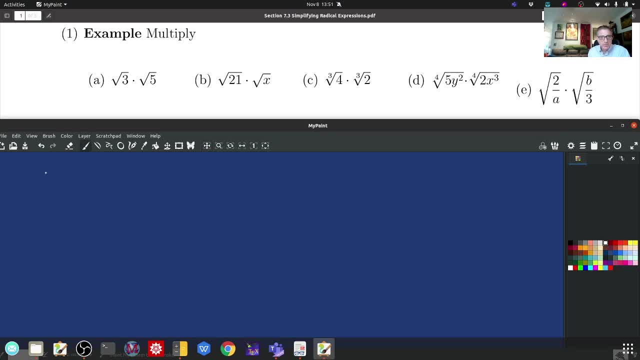 So let's do 1b. Try to mimic this on your own. So again, we are using the square root. So the value of the index is assumed to be 2 times the square root of x is equal to the square root of 21 times x. 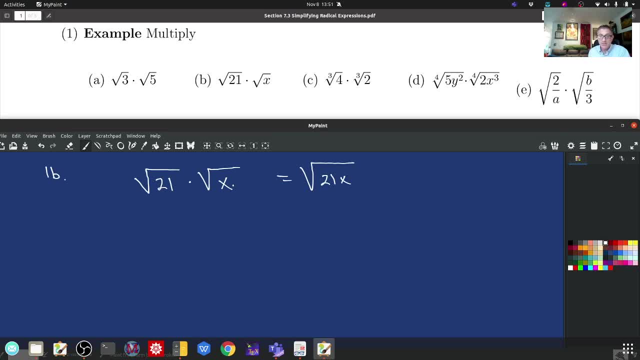 There's nothing that can be done to simplify that, Why Coming over here noticing 21 is equal to 3 times 7.. Now so, writing it out that way: 3 times 7.. If we ever had 21 or some number equal to a list of primes, a product of primes, raise two powers, if we can actually simplify. 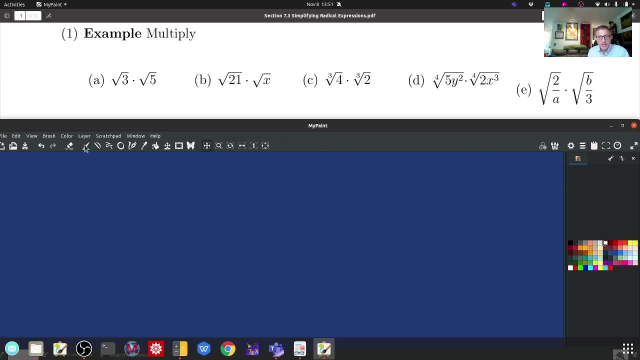 And I think we'll see this right here in our next example. So now our index is 3.. So we can say the third root of 4.. So here we're going to take the third root of 3 times the third root of 2.. 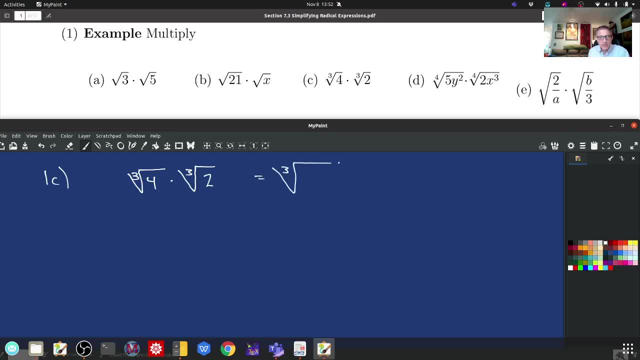 Well, that's equal to the third root of 4 times 2.. But note that 4, we're looking for multiples of 3 in powers. 4 is equal to 2 times 2.. So I'm replacing 4 with 2 times 2.. 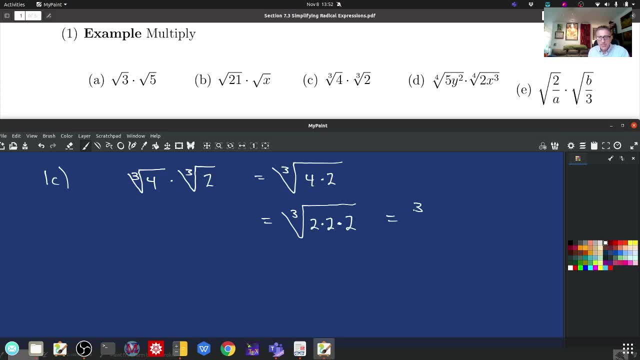 Then I'm multiplying it by another 2.. So this is 2 times 2.. So this is 3 times 2.. So this is 3 times 2.. So this is 3 times 2.. is the third root of 2 to the third, and since our index is odd, 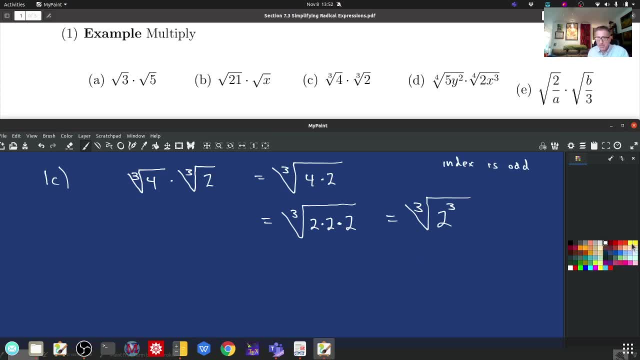 we can actually simplify this even more. now I'm not for sure if they actually do the simplification, but that's equal to 2 to the third raised to the one-third. so that's just equal to 2. so it's not plus or minus, it's just equal to 2, and that's because. 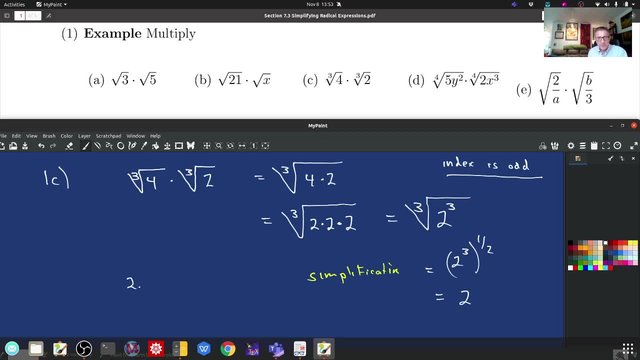 the index is odd. so 2 times 2 times 2 is equal to 8, and that's what it means for the nth root of something to be that value. recall if, going back just to the definition of the square root, so the square root of a number B is some number C such that ST. 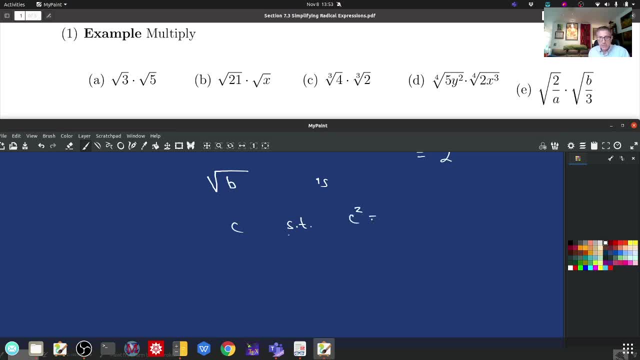 stands for square root of a number B is some number C such that ST stands for square root of a number. B is some number C such that ST stands for, such that C squared is equal to B. so now let's use the nth root, the nth root of B. 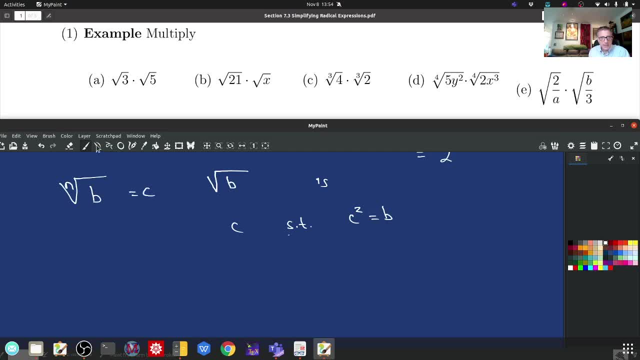 is equal to C whenever, just using a different term other than such that whenever C to the nth power is equal to B. so again, the third root of the square root of 2 to the third. well, if C is equal to 2, then C cubed is equal to 2. 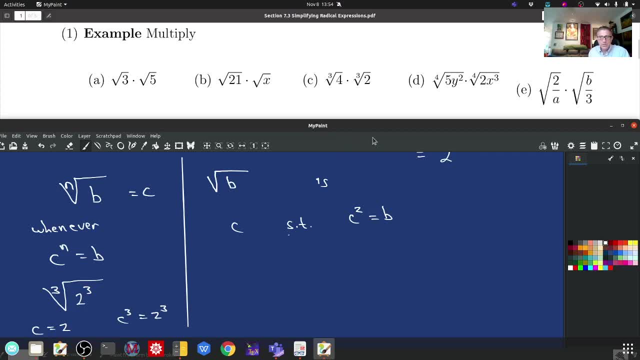 cubed. so the answer there is just plain old 2 plus or minus 2. just plain old 2, 1d. so the fourth root of 1d, so the fourth root of of 5y squared times, again, we have the same index. 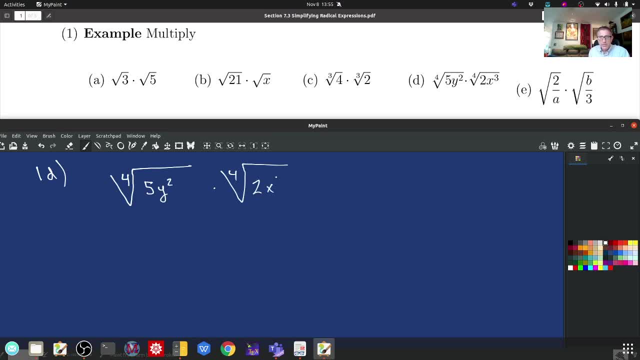 the fourth root of 2x cubed. So the index is even So. we'll keep that in mind. So just using the product rule, that's the fourth root of 5 times 2, which is 10, y squared, x cubed. 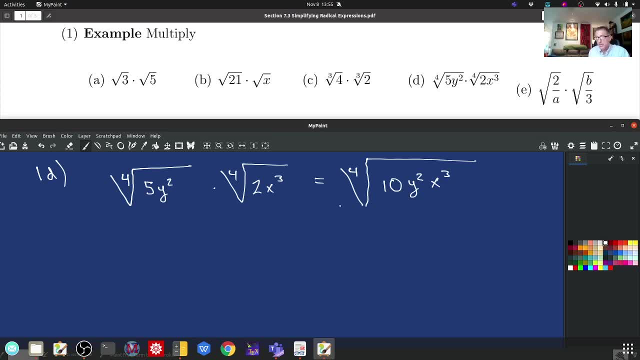 And there can be no simplification. That's all we have Now. the last one: 1e, we have the square root of 2 over a Times the square root of b divided by 3.. So we're literally just going to use the product rule. 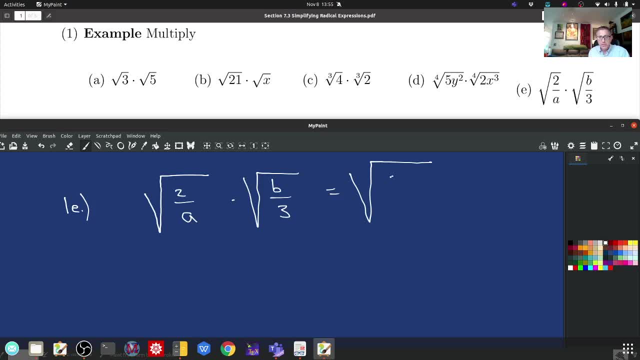 So this is the square root of 2 over a times b, divided by 3.. And make sure when you do this that you extend the radical symbol all the way over so that it includes the numbers under the radical. So the final simplification needed here: 2 over a times b. 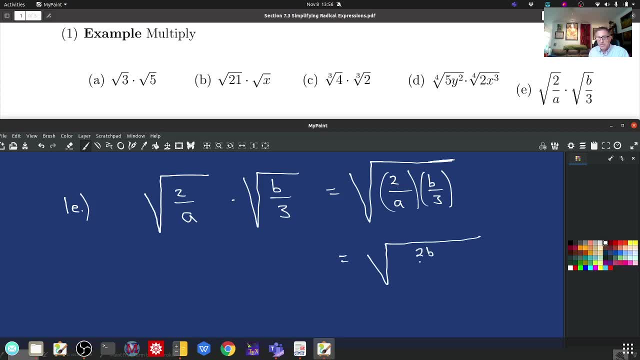 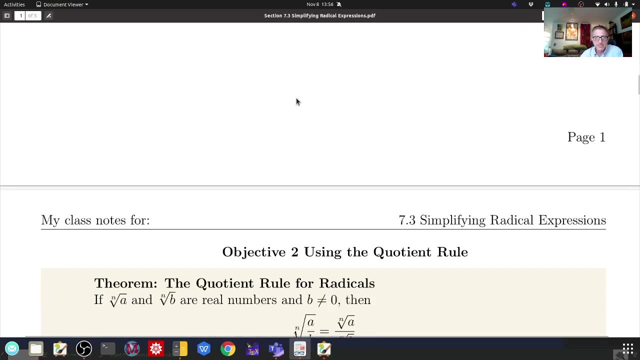 divided by 3, is just simply 2b divided by 3a, And that can't be simplified at all. So let's look at the next page. We're going to be given another rule. It's the quotient rule, And you could have almost anticipated it. 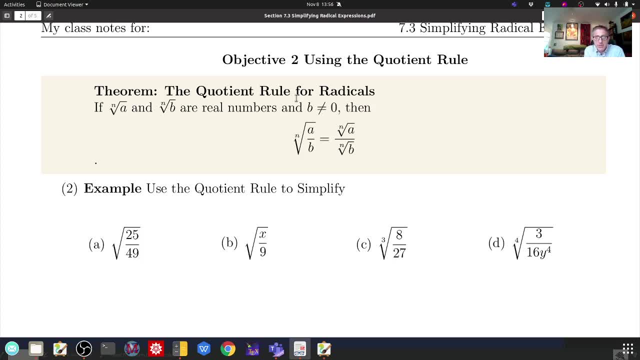 Because really What we're doing is we're using the same rules that we used when the index was 2, when we had the square root, And we're just extending those same rules so when the index has a different value, 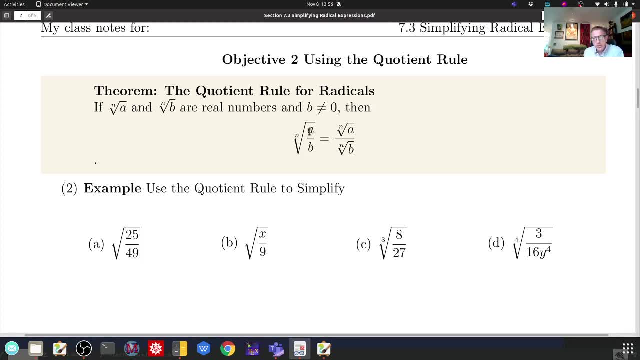 So again we're talking about quotients. So we're talking about some number a divided by another number, b. That means b can't be 0.. We always state that. It's just a habit. It's an important habit in math. 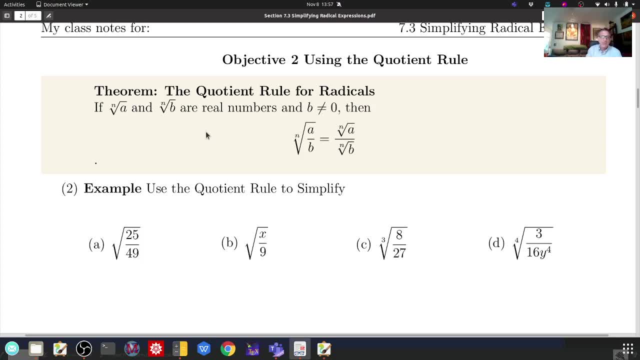 I've actually seen papers written by non-math mathematicians- philosophers usually- that try to prove something using math And they forget to check if their denominator is 0. And they prove things that don't follow because they don't check And indeed the conclusions they actually arrive at don't follow. 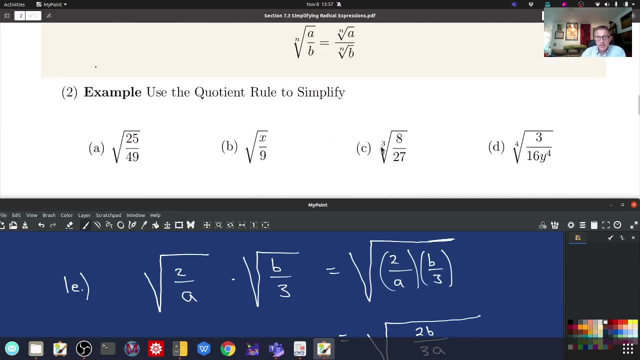 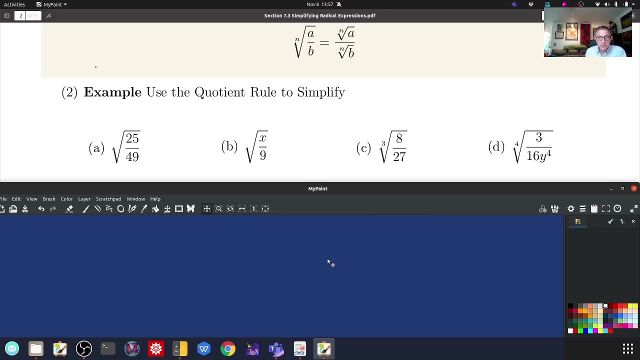 because explicitly the denominator is equal to 0. And you can't do that- Mathematicians would probably do that- trained differently, that's for sure. by the time you get to grad school you're trained quite a bit to always check to see about division by zero. so the square. 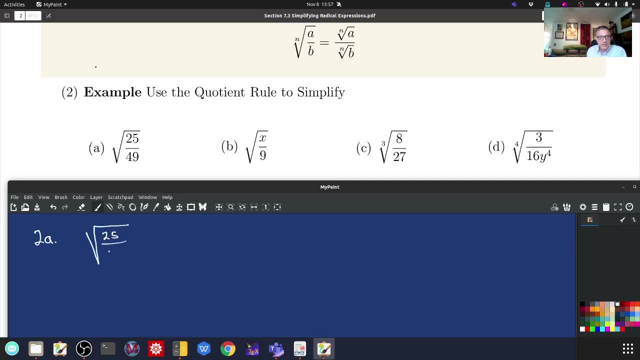 root of 25 divided by 49, again just using the quotient rule, don't you? which which you already know, because the index here is 2, so the square root of 25- so we always take the positive root- is 5 and the square root of 49 is not 9 but 7. 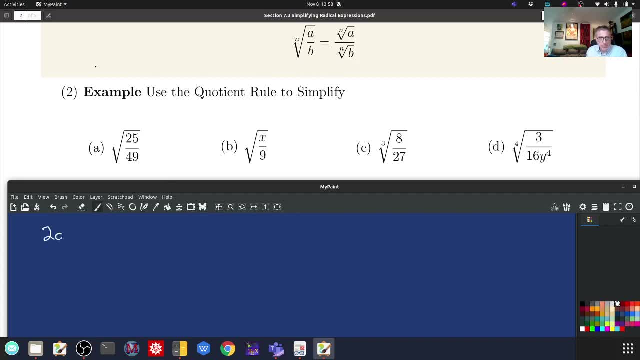 so this is? this is pretty simple, pretty basic. the point with you taking this at home is you can't let yourself get bored. you can't let yourself be distracted. that means, when you sit down and you watch these lectures, you've got to do it at a time that works for you. so this is just a direct application from 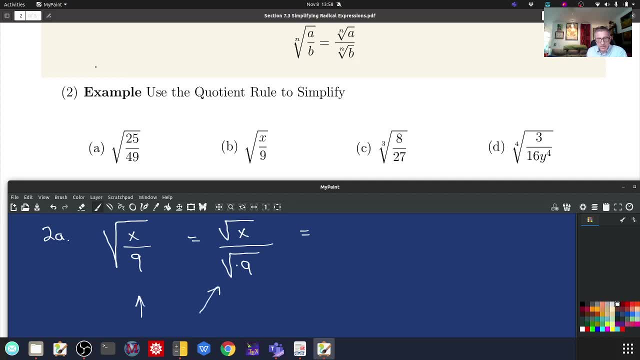 this step to this step. here it's just a direct application of the quotient rule. but I can simplify. the square root of 9 should go ahead and do that. square root of nine is just three, so the cube root now of eight divided by 27: well, that's the cube root of eight. 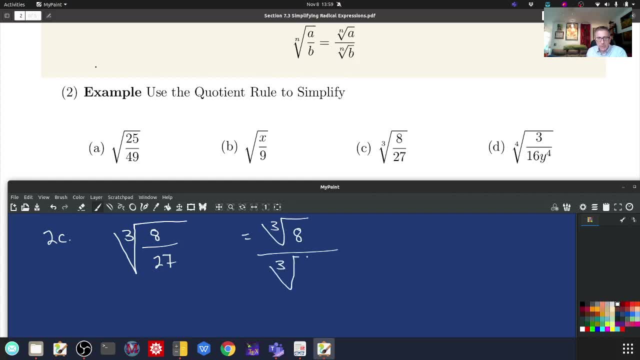 divided by cube, or the third root of 27. either way is fine. now, in our previous example, we just learned that 8 is equal to 2 to the third, so I'm going to rewrite 8 as 2 to the third and, as it turns out, 27 is 3 times 3 times 3, so it's 3 to the third. 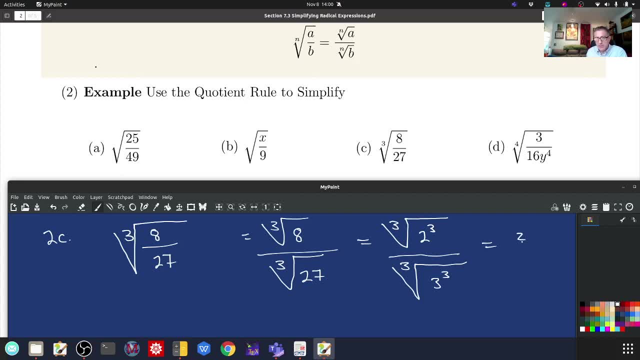 so that's equal to 2: 2d. the fourth root, that's a. even so, we would always just take the positive answer, if there is any. you'll see what' gonna happen here. so that's equal to the 4th root of 3.. That cannot be simplified. That's an irrational number. The bottom is: 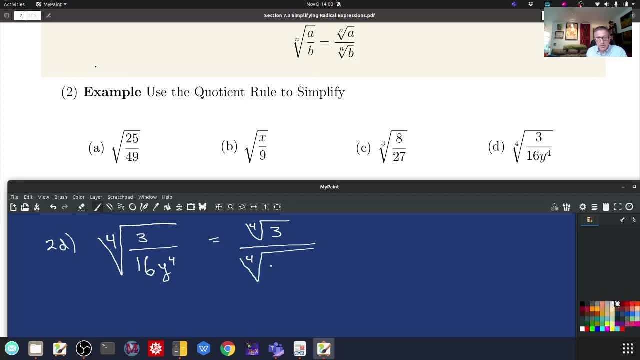 the 4th root of 16y to the 4th. So let's think about what is 16.. 16 is equal to 2 to the 4th, So that's times y to the 4th. So bear with me, I'm doing this in steps, You're okay. 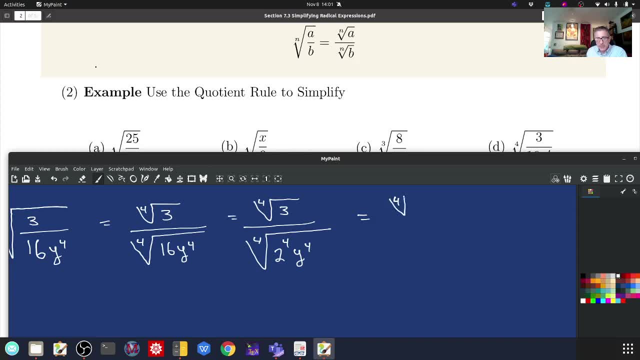 to skip some of these steps. Again, we've already stated that the numerator cannot be simplified, But using just the regular exponent rules, 2 to the 4th times y to the 4th is 2 times y. So we're almost ready for one last simplification. So again, this is the 4th root of the square. 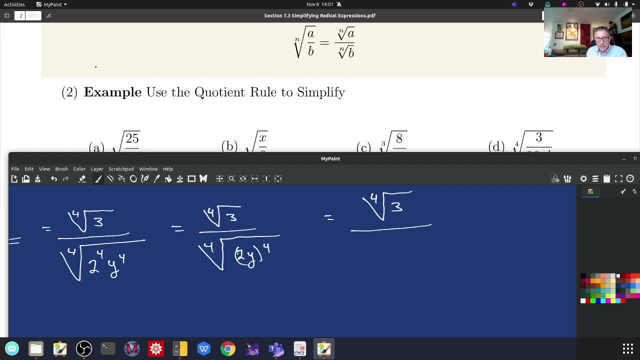 root of 3.. So, since this is the 4th root of something raised to the 4th, when I take it outside of the radical, I have to make sure it's positive. Now the problem is here is, I don't know? 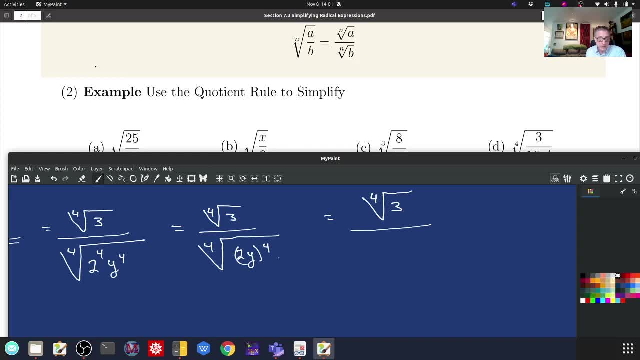 I don't know whether y is positive or negative. If it's negative, when it's raised to the 4th, it's going to become positive, So I don't have to worry about a complex root here. So, in order to assure that we get a positive value, we put it in absolute value signs, And there is one. 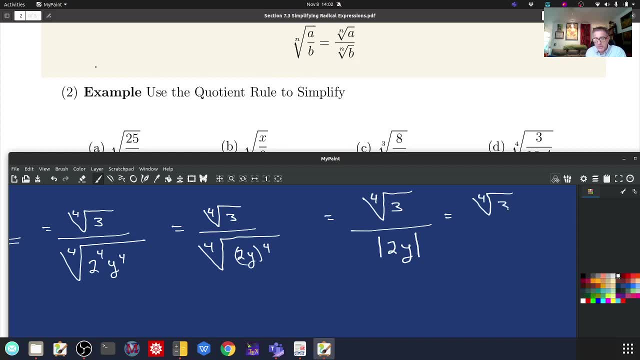 last simplification here, And these are simplifications that I think my math is going to be able to do. My math lab will make you do So. since 2 is always positive, I can take it from in between the absolute value signs. So it's 2 times the absolute value of y, And that's. 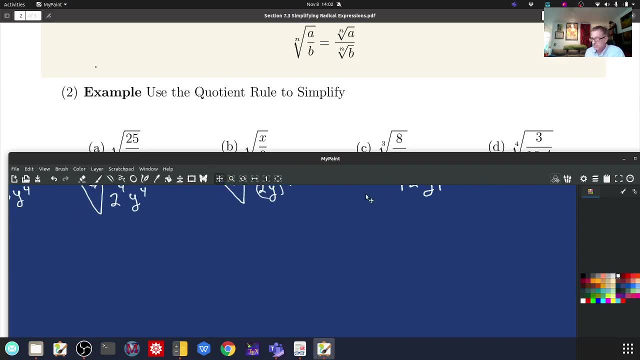 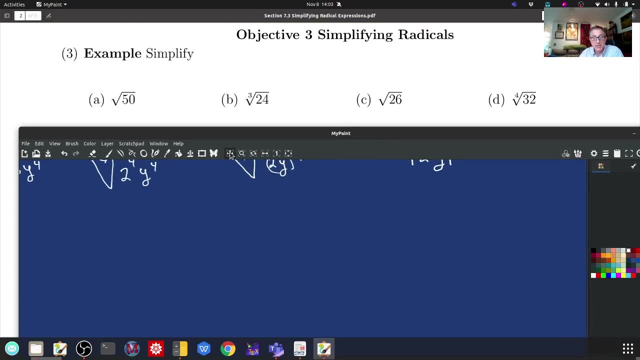 the end of that one. So let's do some more simplifications. So these simplifications are going to require some factorizations of the numbers inside them. So let's look at 3a. So by the numbers inside I mean the numbers under the radical. So let's come over here and let's factor 50. Well, 50 is. 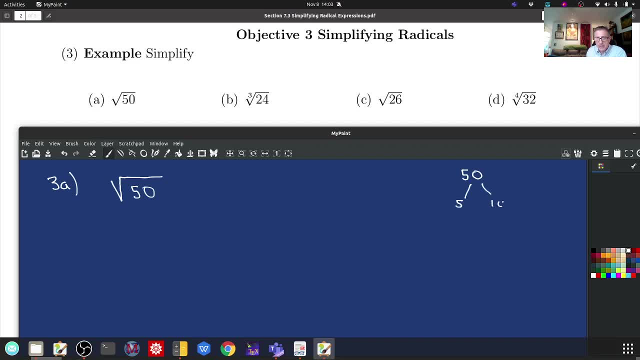 clearly 5 times 10.. So let's do some more simplifications. So let's do some more simplifications. So 50 is equal to 2 times 5 times 5.. But another way of writing that is 2 times 5 squared. So that's. 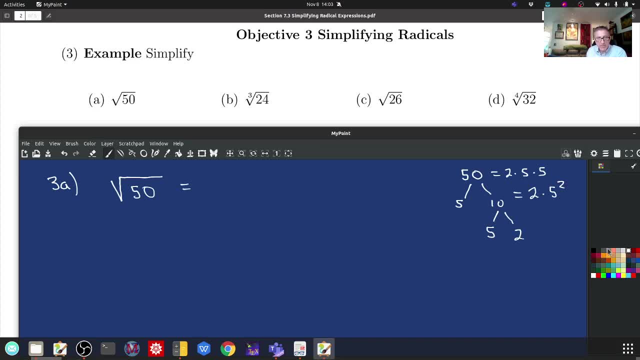 what I'm going to write over here. Notice, remember, my unstated index here is always 2.. So I'm taking the number of times 5 squared, And I'm going to take the number of times 5 squared And I'm going to. 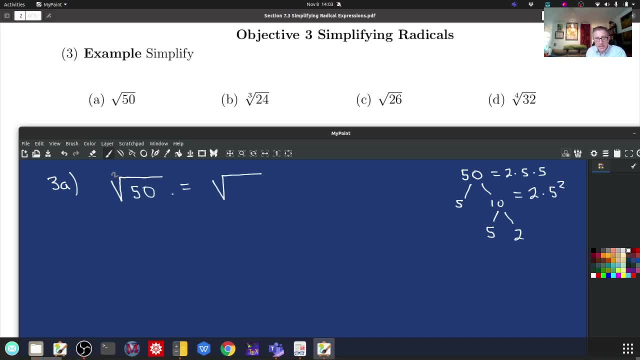 taking the square root. I'm not writing 50 as it is, but rather this way: 2 times 5 squared. So here we have. since my index is 2, I have a power raised to an even power, something that is divisible by the. 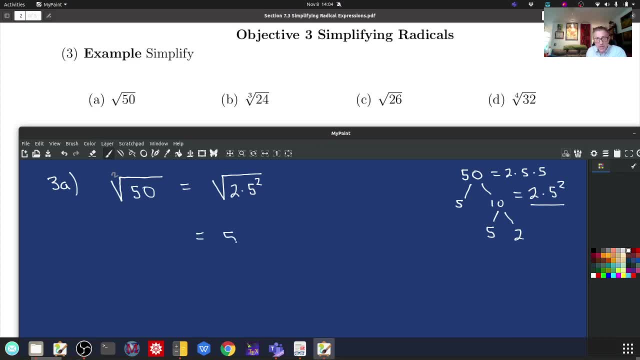 index. So I can take this whole component 5 squared outside, But the price is going to be 2 times 5 squared, So I have to pay to move it on the outside of the index or outside of the radical symbol is to divide its existing power by the index power, which is 2.. So that equals to 5 raised to. 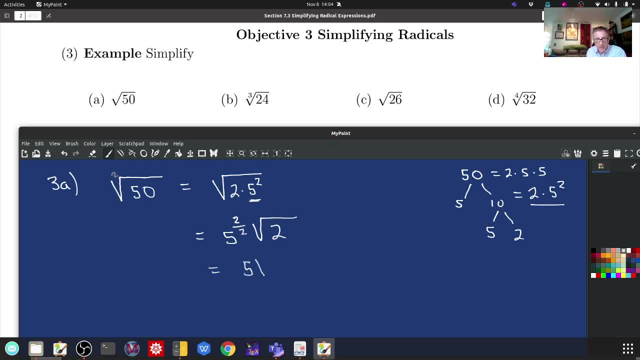 the first power times, square root of 2.. So that's kind of how we're going to do these 3b. So here we have the third root of 24.. So the first thing we have to do? we don't really know, can it be? 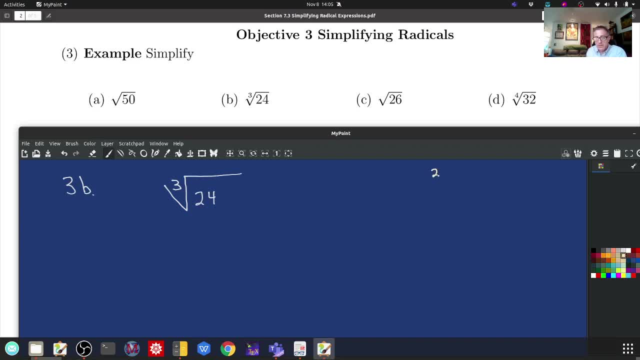 simplified or not. Let's come over here and let's factor 24.. I always just start with the easiest thing, to divide it by the thing that pops to my head first, And in this case that's going to be 2.. You could use 6, that. 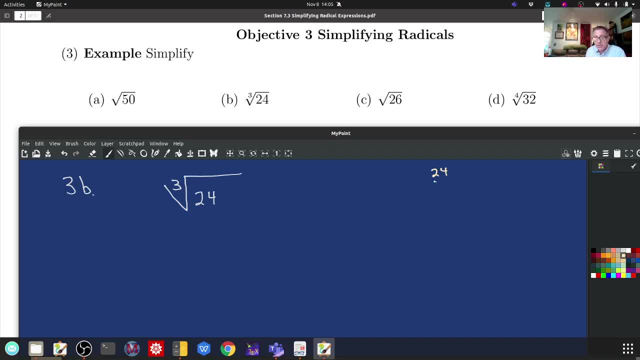 would be okay, But I'm going to take the number of times 5 squared. So I'm going to take the number of times 5 squared. That's going to be okay as well, but it's going to be 2 for me, So that's 2 times 12.. Now, 2 is prime, so that 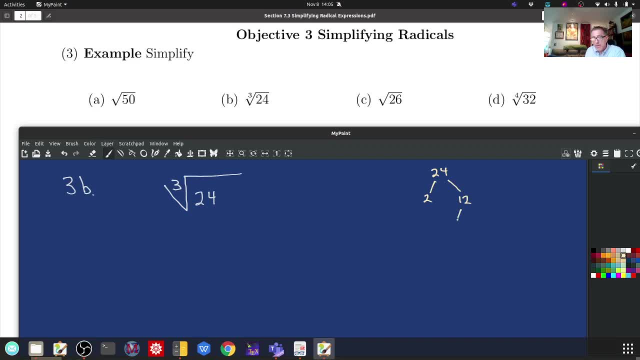 branch of the tree is done. However, 12 can also be divided by 2, and I get 6.. Ah, but 6 can also be divided by 2, and I get 3.. So 24 is equal to 2 times 2 times 2,, which is 2 to the third times 3.. So I'm going to 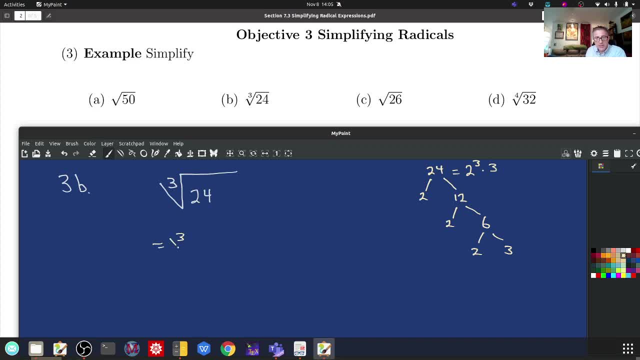 write this as the third root of 2 to the third times 3.. So here I have an exponent under the radical that is divisible by the index. So that means I can move it out from underneath the radical. The price for doing that is I. 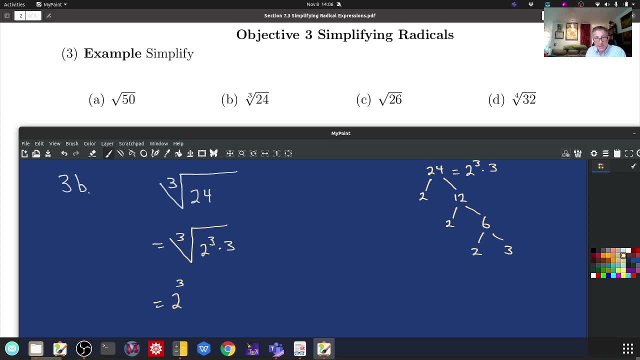 have to divide the existing exponent, which is 3, by the index value. The 3 has to stay underneath there. But 2 raised to the 3 divided by 3 is just 2 raised to the first power, which is just 2 on the. 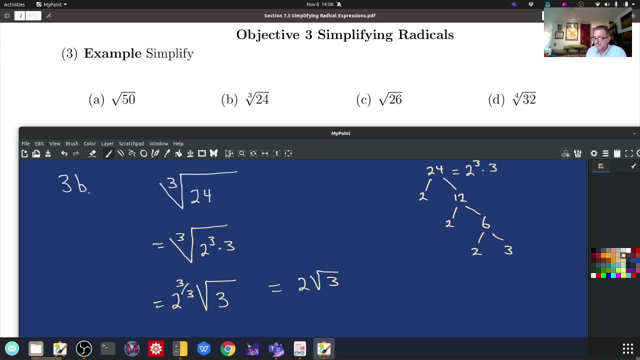 square root of 3.. And sorry, I need to bring down the fact that this is my radical index is 3.. It's really easy to forget to bring that down. We're habituated to just write the square root symbol. but that's an important bit of information And in a way it kind of is a call to say, hey, stop using the square root symbol, use the square root symbol and the index, but that's never going to happen. 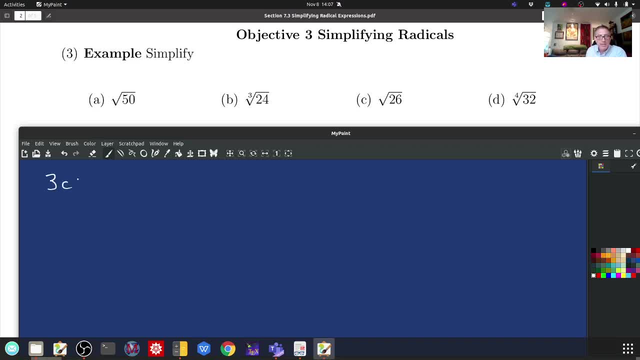 Mathematicians are humans too, and they get set in their ways, just like humans, all humans. So again, my index here is 2.. So this is 26.. So what I'm going to do is come over here and let's factor 26.. So again, the first thing I see is it's divisible by 2. It's 2 times 13.. So I don't have any powers. Both of these are not two powers that are evenly divisible by our index, which is 2.. So done, There is no further. 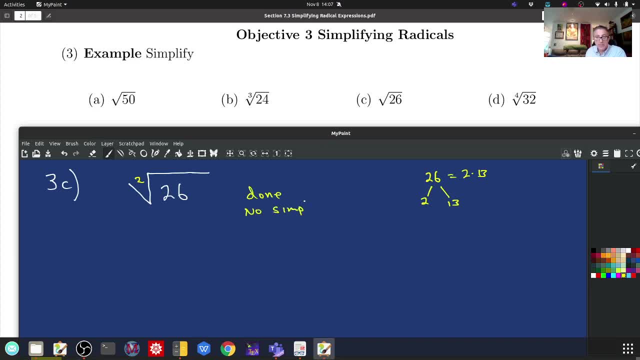 simplification. It is as simplified as it can be. So now our index is 4.. We're going to do the 4th root of 32.. So let's come over here and factor 32.. Divide it by 2, that gives me 16.. 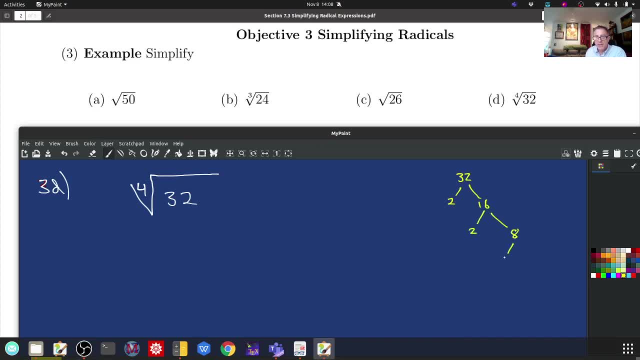 I'll divide 16 by 2, that gives me 8.. Divide 8 by 2, and it gives me 4.. Divide 4 by 2, and it gives me 2.. So these are all primes. So 32 is equal to 2 raised to the. what power? 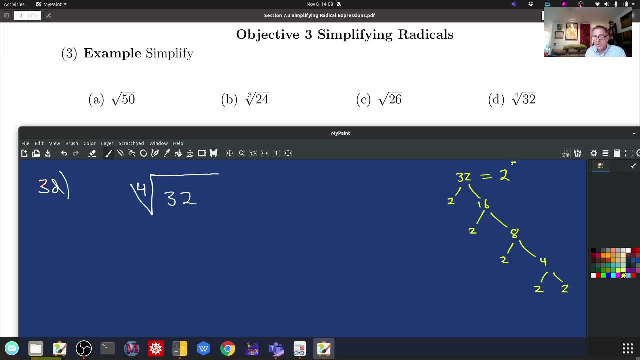 1, 2,, 3, 4, 5.. 2 to the fifth. So this is equal to the fourth root of 2 raised to the fifth. Now here's the thing: If you have a power, an exponent, 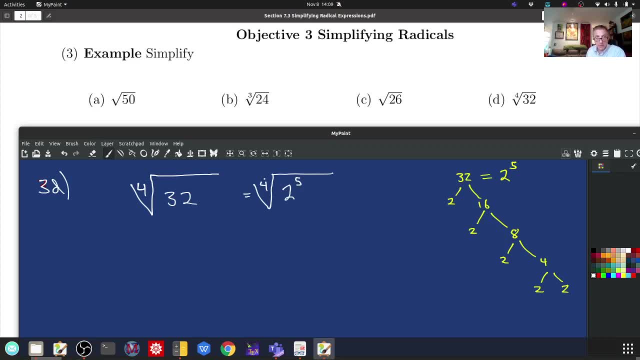 under the radical that is larger than the index, then what you need to do is to subtract numbers until you get a number that is evenly divisible by the index. So what I'm going to do here is I'm going to write: 2 to the fifth is 2 to the fourth times 2,. 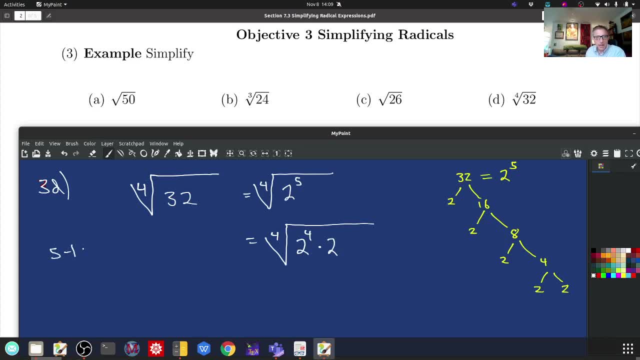 because 5 minus 1 is equal to 4.. So I have to do 2 to the 5 minus 1 times 2, and that's equal to 2.. So I have to do 2 to the 5 minus 1 times 2,. 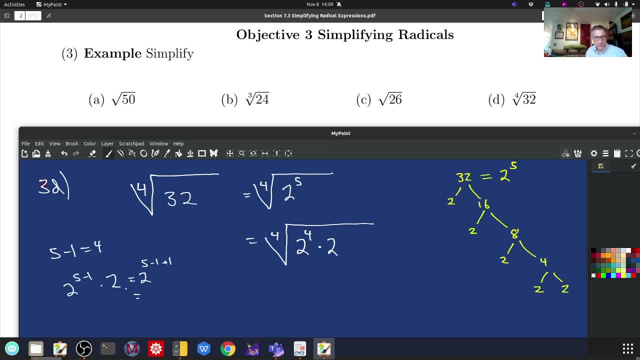 plus 1, which is equal to 2 to the fifth. So I have my equality. So now what can I do? If you didn't understand what I did over there, it's a little math trick that we do If you expect sometimes to really like math and major in math. 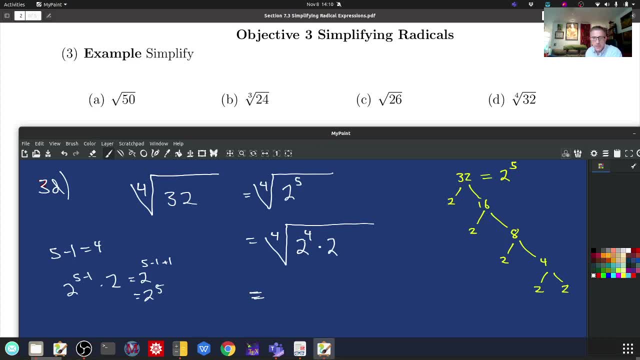 it's for those people, For everyone else, just ignore it. So what can I do? The exponent here is greater than 1, and it's divisible by 4.. So I can move 2 to the fourth outside. Now to move it out from underneath the radical symbol. 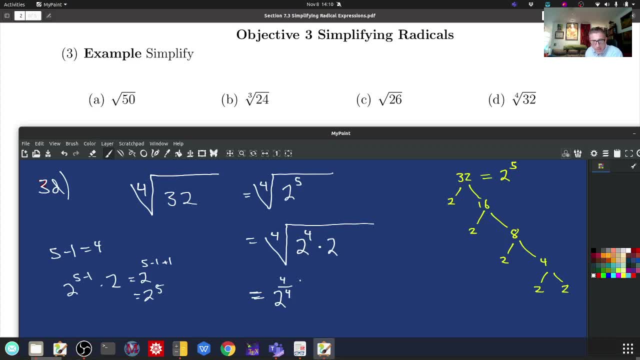 I have to divide its power by the index And of course this factor of 2 has to stay underneath. So 2 to the 4 divided by 4 is just 2.. Remember, I need a fourth root right there. So it's 2 times the fourth root of 2.. 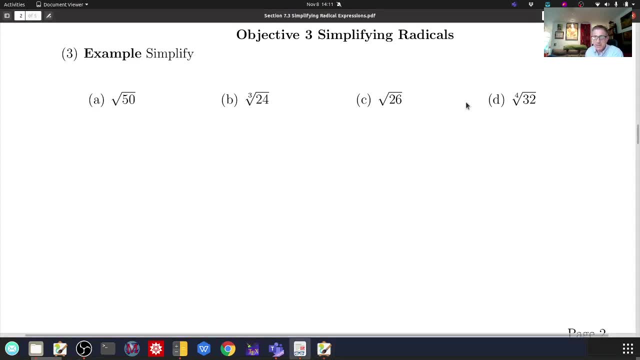 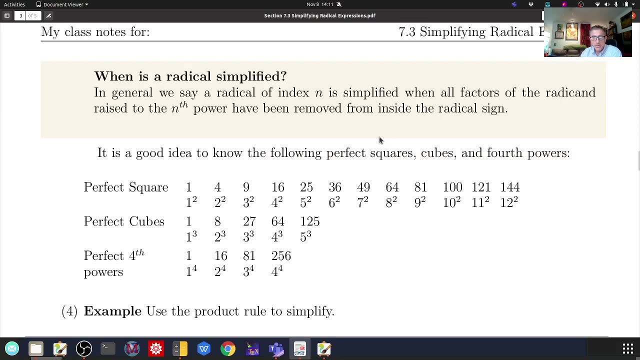 And so just remember to copy down your index. It's a really easy thing to forget, But without that index there, the default is that you're thinking that the index is 2, but it's not, It's 4.. So when it's any number, that's not 2,. 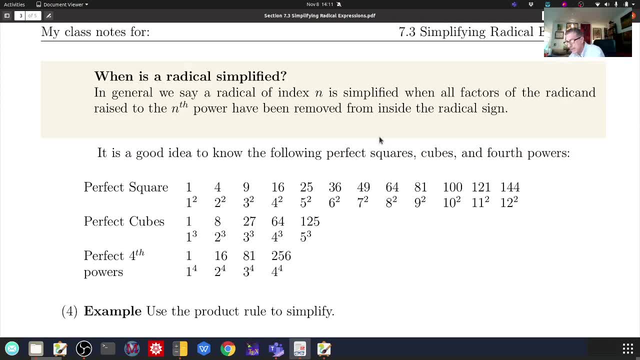 we are obliged to write it down. So here is something that you want to. this is a page you want to include in your notes. So when is a radical simplified? So in general, we say that a radical of index n is simplified when all factors of the radicand raised. 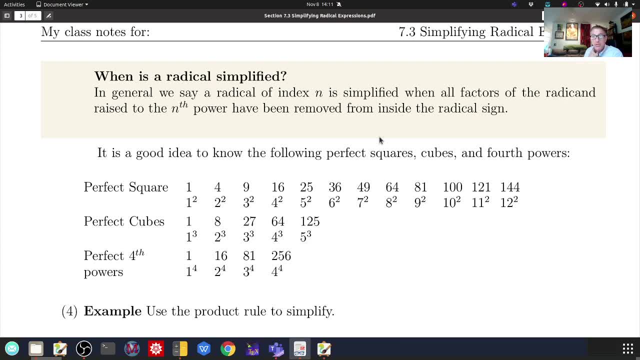 to the nth power have been removed from inside the radical sign, Every factor. So that's what we've actually been doing And here's kind of the end. So that's what we've actually been doing And here's kind of the more technical definition. 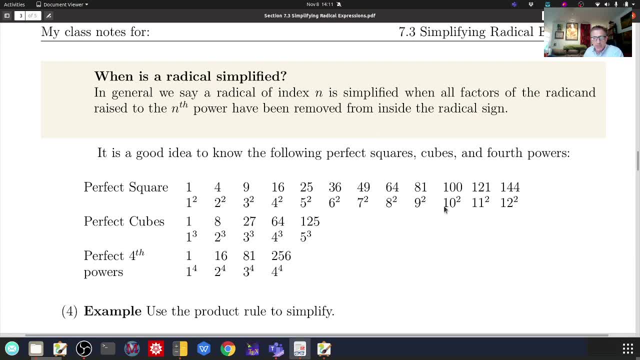 So it's a really good idea that you remember this list of perfect squares. 2 squared is 4.. 12 squared is 144.. You already probably memorized these in high school. When I was in high school, we didn't go beyond 10.. 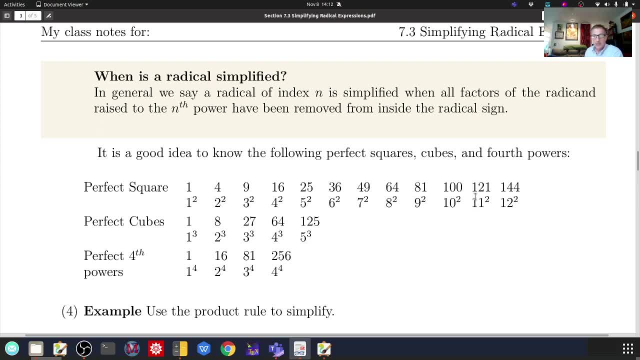 We just had to remember 10 squared And it's kind of embarrassing, if I'm not mistaken for a more sophisticated way of doing this. So we're going to have to go beyond the multiplication tables. We quit at 10.. We didn't have to go beyond 11.. 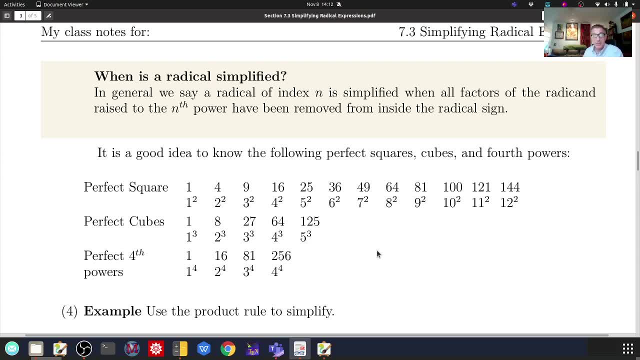 I mean we didn't have to go to 11 or 12.. I think it's standard practice now that you go all the way to 11 and 12. But I could be wrong. It's been a long time. Perfect cubes. 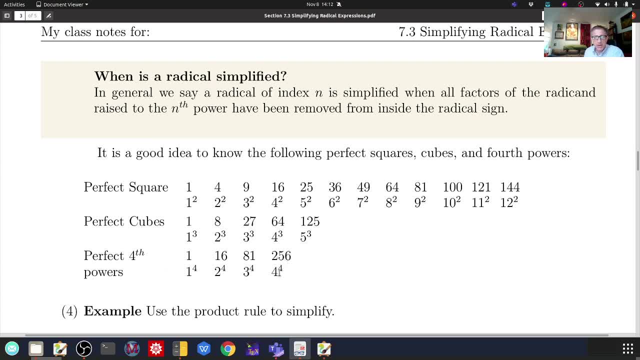 1,, 8,, 27,, 64,, 125.. And perfect fourth powers. So the fourth power of 256 is 4.. The third, Sorry, The fourth root of 256 is 4.. The fourth root of 81 is 3.. 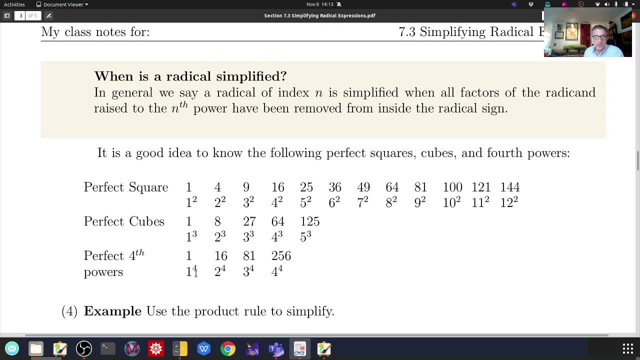 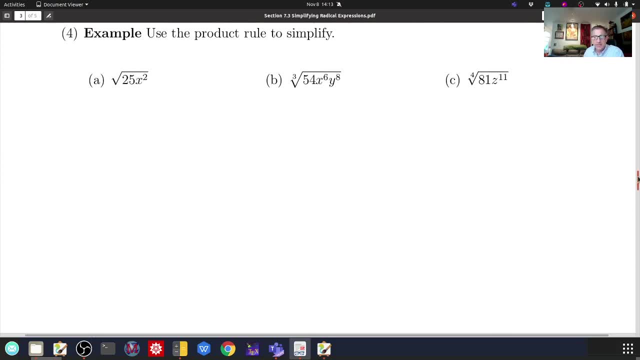 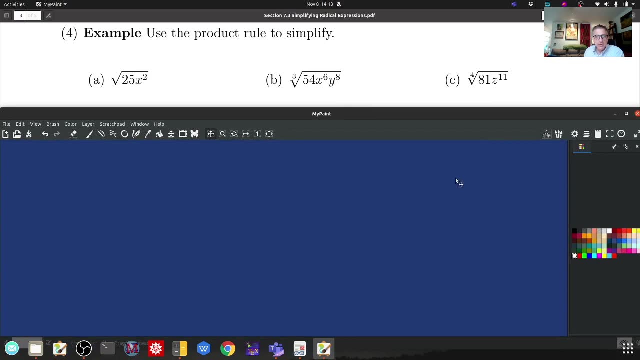 The fourth root of 16 is 2.. And the fourth root of 1 is 1.. So we're going to use that information to simplify Again. the only real game we have in town is the product rule, So I'm adding absolute value signs. 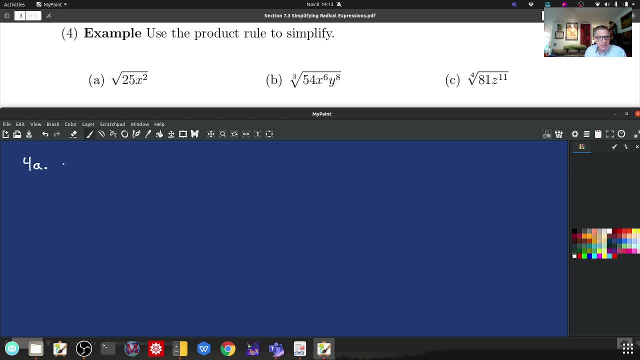 It seems to me, one of the objections I have to this particular book is that they teach you about the absolute value sign, which I introduced to you in either the lecture before this or the one right before this, And then they get to 7.3 and they forget all about it. 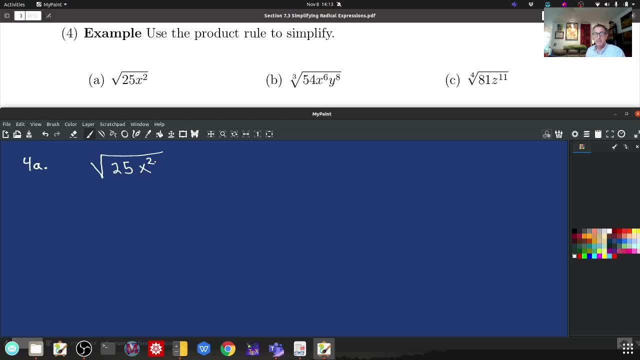 Or they hedge their bets and say: pretend all values of x are positive. So if all values of x are positive, you don't have to worry about the absolute value sign. That's just malarkey. So 25, we should know already- is equal to 5 squared. 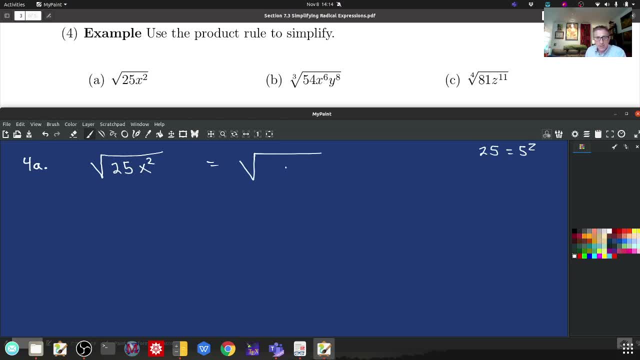 So remember, our unwritten index is 2. So that's 5 squared times x squared. So that's equal to the square. So that's 5 squared times x squared, Square root of 5x squared. So when I move this out from underneath the radical sign: 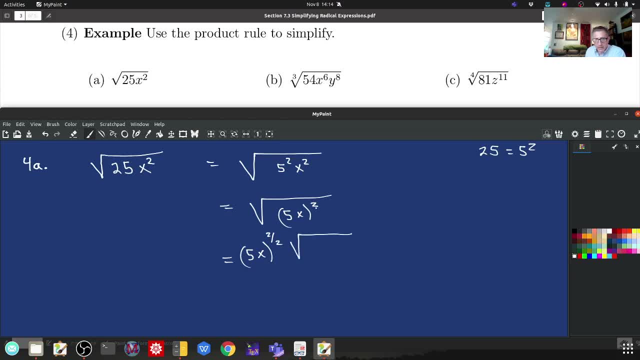 I have to divide the existing exponent, And when I move it out from underneath, we leave a factor of 1.. Now the square root of 1 is 1.. So I really don't even have to bother to write that, But I'm just going to show you it didn't disappear. 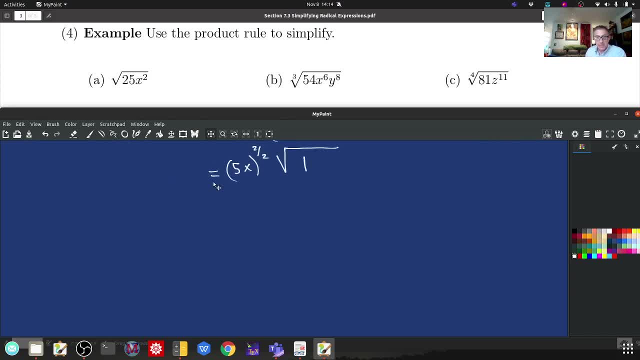 There's no magic. I'm still using the exact same pattern before. The only difference here is when I've moved it out. I don't know if x is positive, So technically this is equal to 5 raised to the first power times, the absolute value of x times 1.. 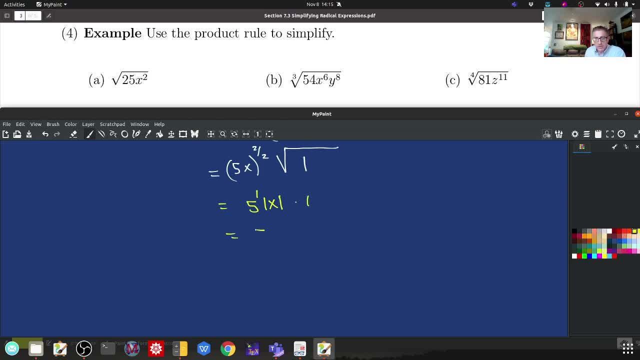 Because the square root of 1 is 1.. So its actual answer is 5 raised to the absolute value of x. But I think in your homework they state something along the lines: assume all variables. Now you all have to check me on this. 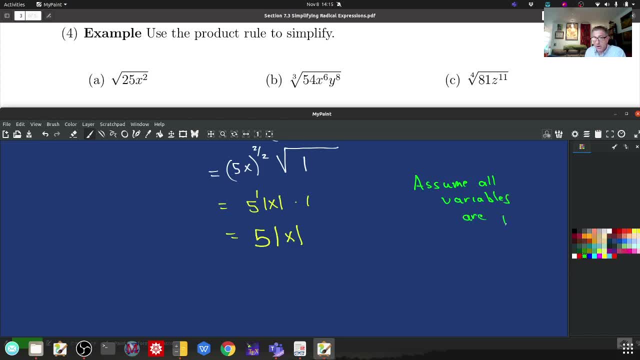 You see the homework- are positive. So if I already know that x is positive, then the answer that you would enter in here would just be 5x And you wouldn't need the absolute value sign, because the absolute value sign doesn't do anything to a number. 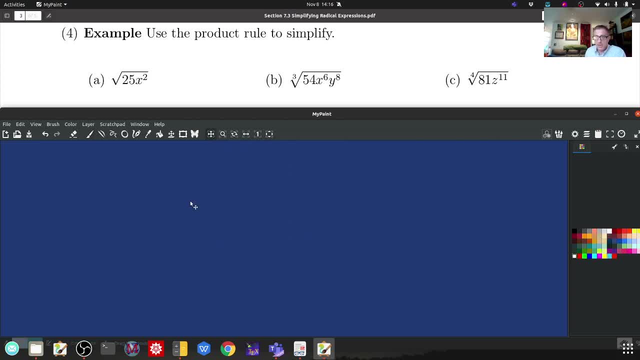 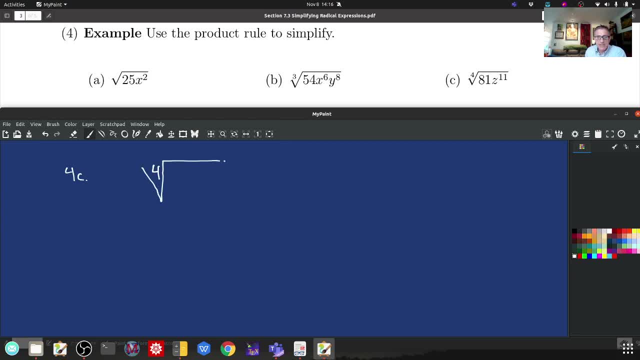 So we're on fourth roots now. So that list of fourth roots will be really really good for you. So 81 times z to the 11th. So I hope the obvious thing that you're going to do here now is rewrite 81.. 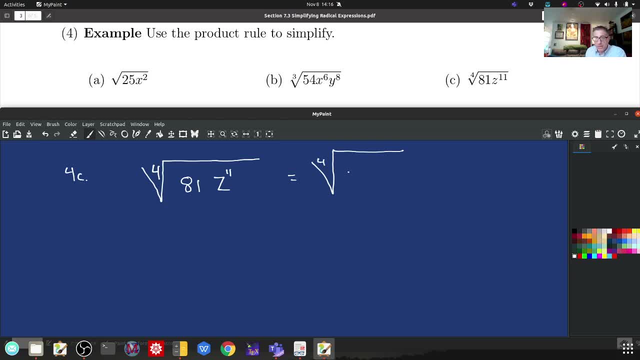 Just look at the notes I just gave you. Is 4 raised to the fourth power? But what about z to the 11th? I need to subtract some values of 11 so that I get to something that is divisible by 4.. 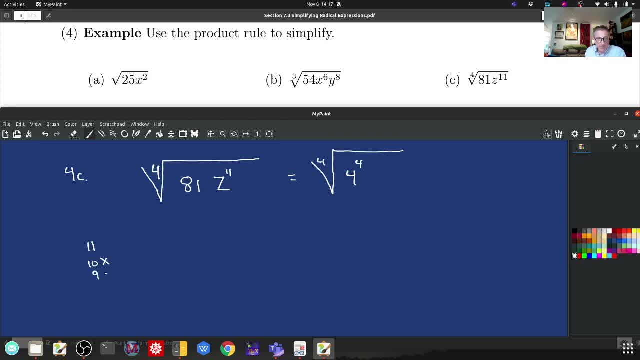 So 10 is not divisible by 4.. 9 is not divisible by 4.. But 8 is. So I'm going to write this as z to the eighth times z to the 8th. So I'm going to write this as z to the eighth times z to the 8th. 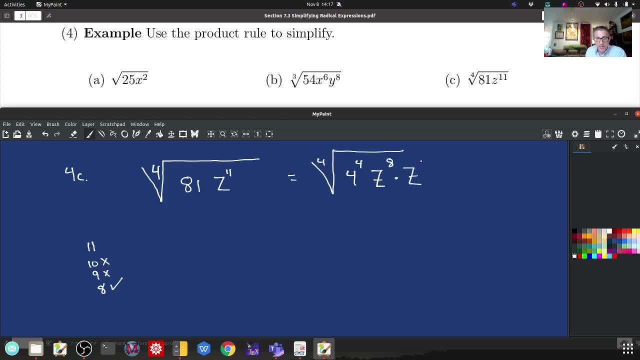 So I'm going to write this as z to the 8th times, z to the 8th Q, as 8 plus 3 is 11. now what do we do we take these factors that are raised to exponents that are powers of 4? we can take them outside. in each case, we have 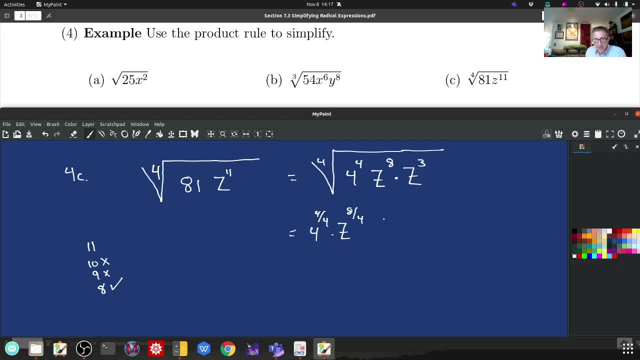 to divide the existing exponent by the index form. again, I have the fourth root here in Z cubed. so this is equal to 4 raised to the first power and this is equal to Z. 8 divided by 4 is squared and that's going to be. you don't have to put. 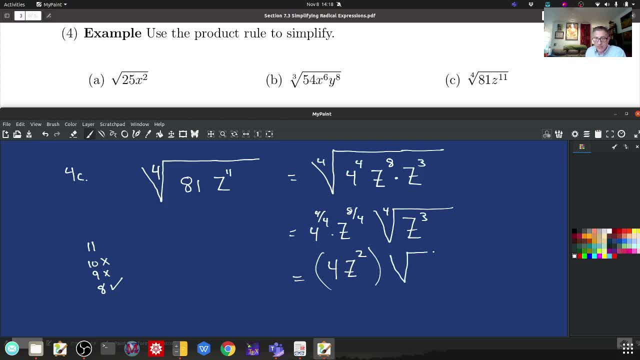 parentheses there times the fourth root of Z. cute, I messed up, didn't I? so for those of you who are waiting for me to catch my mistake, I was thinking I was concentrating on the power there. 81 is equal to 3 to the fourth. I just 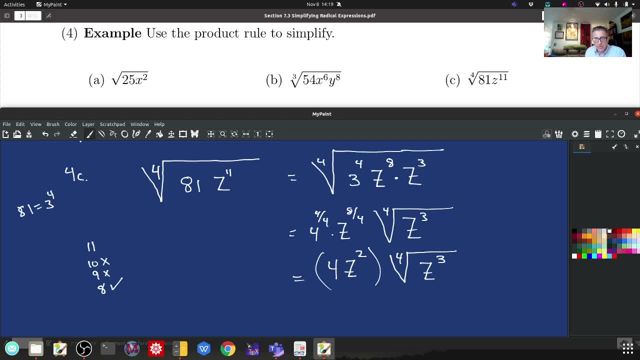 wrote forward to the fourth, focusing on the fact that it was raised to the fourth. sorry about that. so let's go through and just replace everything 3z squared. now I don't have to worry about absolute value signs and, like I said, I don't think the book makes you worry about absolute. 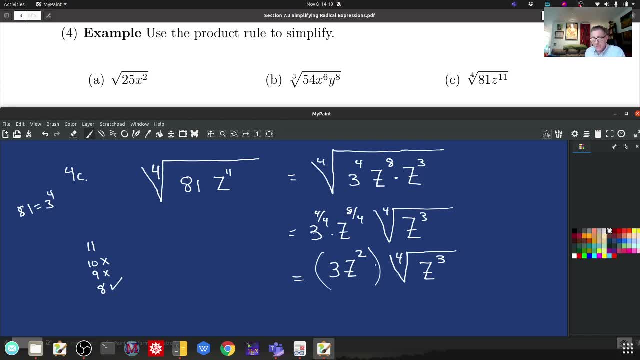 value signs, but in this case I wouldn't need anyway, because no matter whether Z is positive or negative, z squared is going to be positive. so the absolute value of some number squared is just Z squared. they're always identical. so I'm going to go over the 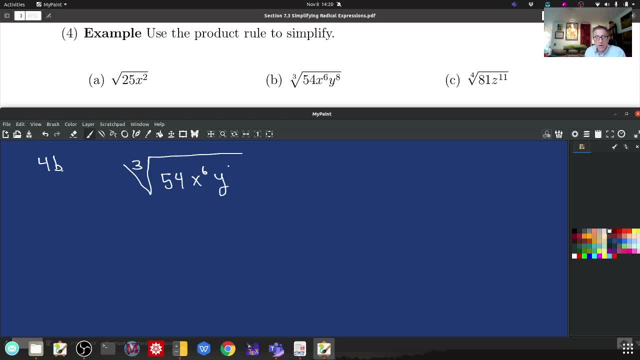 zeros and the zeros are the same. so I'm just going to move here and do the third can do to change that. so it's divisible by 3, but I need the factorization of 54. well, 54, I'm going to divide it by 2 and that's equal to 2 times 27, and let's 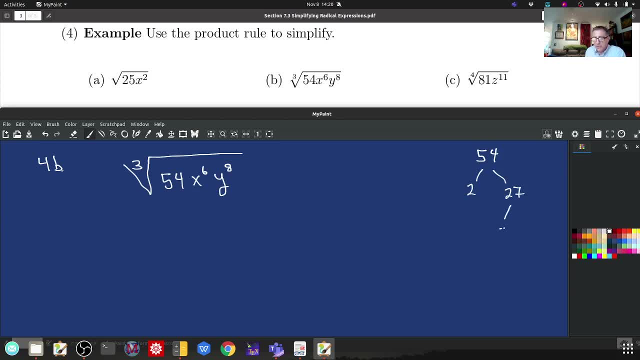 look at our third roots: 27 is equal to 3 to the third. so this is equal to 3 to the third times 2. so that's exactly what I'm going to do when I start my simplification. 54 is 2 times 3 to the third, times X to the sixth. so what can I? 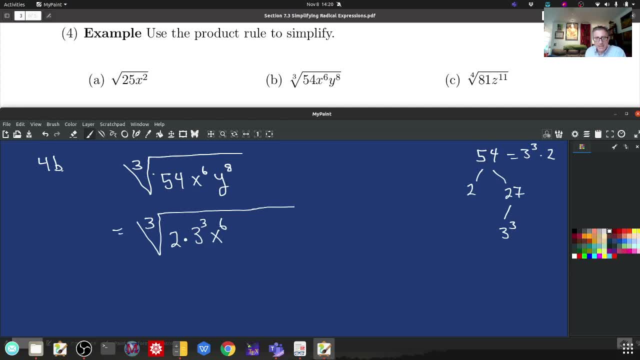 do to get Y to the eighth. well, eight is clearly greater than three. so that means I can do something. if I say, subtract two from eight, I get six. so I can write Y to the eighth is Y to the sixth times Y. so I'm just going to dispense with the absolute value signs. 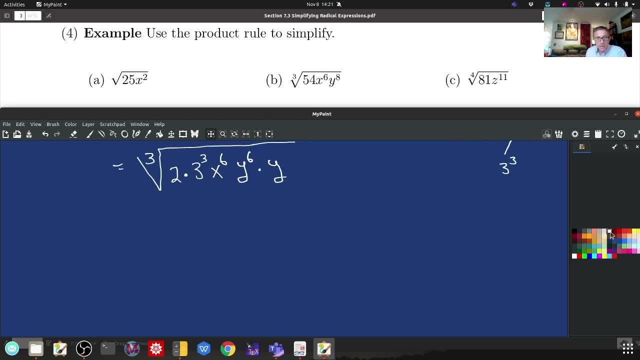 from now on? and what can I do here? 3 to the third can come out, but its existing exponent has to be divided by the index times. y to the sixth. that can come out, but it has to be divided by three, the index. I forgot. x to the six, x to the six can. 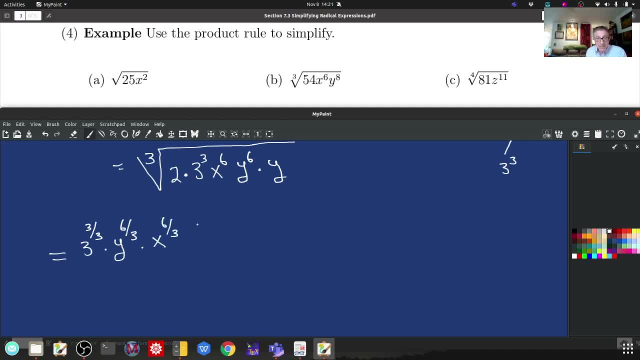 comes out can come out, but it has to be divided by three. and what's left in there? just my two and my y. I just have to remember to write my index here. so three to the first power is three. y to the sixth, divided by three, is y squared. x to the sixth, divided by three, is x squared. so that's. 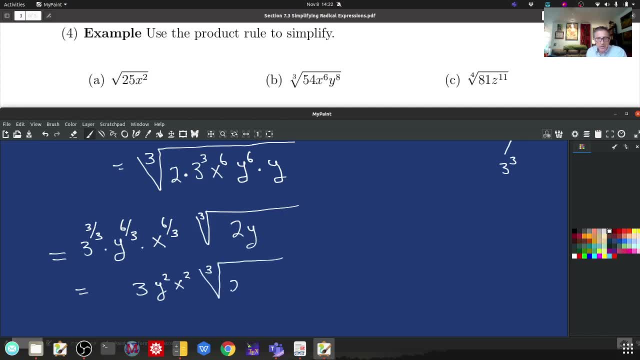 the third root of 2y and they would probably- and it's annoying and you all know more better more about that to than me- it would probably want you to write this as 3x squared y squared times the third root of 2y: they. 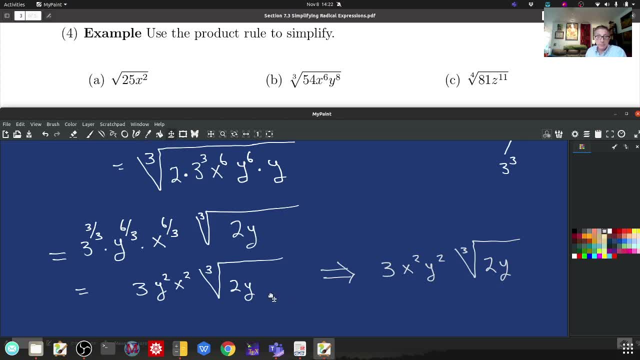 should not require that we have plenty of symbolic tools that can easily determine the y squared times. x squared is the same as x squared times y squared, and bonus points for anyone else who might see yet one further simplification of this, going all the way back to our exponent rules. it seems like it's been forever now this. 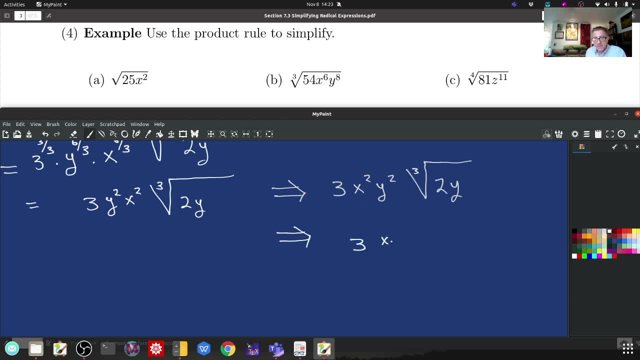 is the same thing as 3 times x times y. using the power of a product rule, squared times the cube root of 2y. I think they're okay with this one. I would certainly be okay with that one on a exam. I would not expect that final step to that final step is it's more of a kind of your subject. 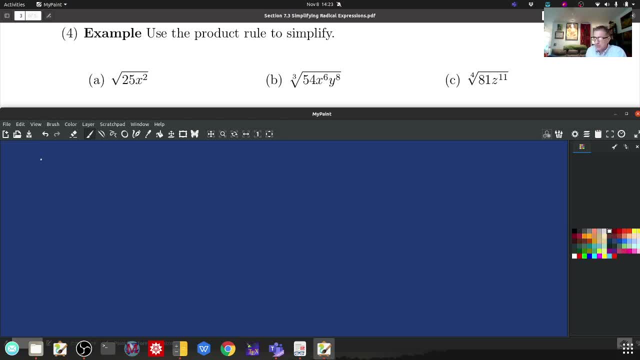 subjective preference, and this is one thing I'll tell you. I will never count. count off for a subjective preference. now you've already experienced the fact that I have required you to do some work using a specific method I taught you. now that wasn't because of my subjective preference, it's. 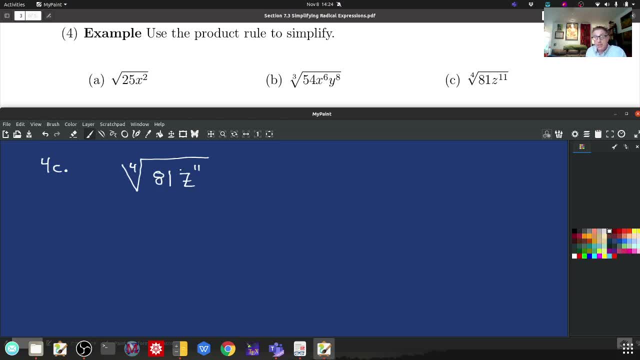 because online symbolic help cannot does not do it that way. so by me forcing you to do it that way, I'm assured you're not using something on your screen that I can't see and, in essence, using illegal tools and getting grades that you shouldn't be getting because you didn't study. 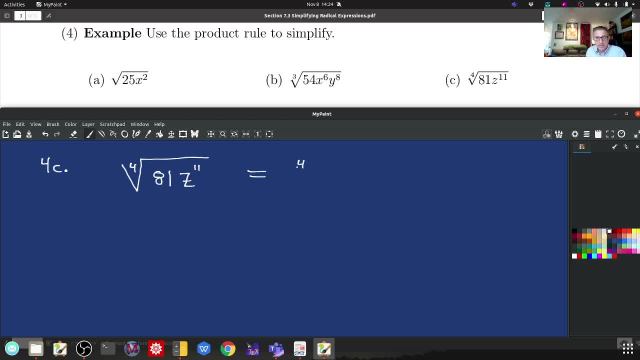 to get those grades. I would be happy to give it to your computer. so 81 again is 3 to the fourth by the list we just saw, and z to the 11th I'm going to write is z to the 8th. seems like I just did this. 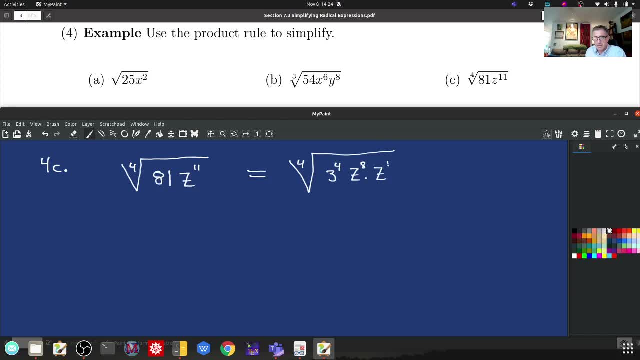 one did. I just do this and I'm getting deja vu here. so, any rate, this is three to the four divided by four times z to the 8 t by 4 times what's left inside. it's not 11, it's 3. sorry, talking too much here. 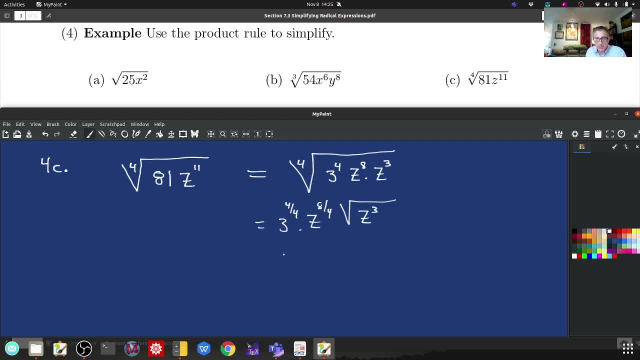 I'm trying to figure out if we really and truly just get to this one- and yes, we did so. that's 3 z squared times the fourth root of z cubed. I don't know why I did that one twice. Whatever, maybe it's deja vu. 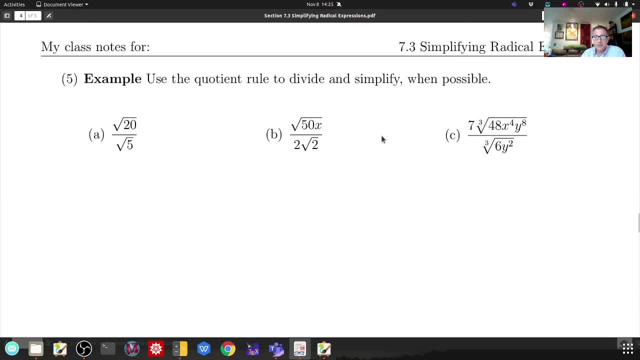 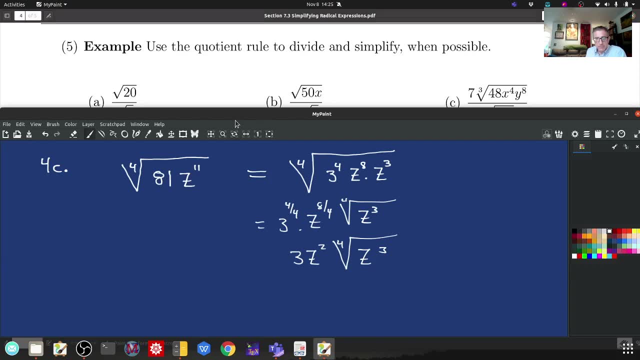 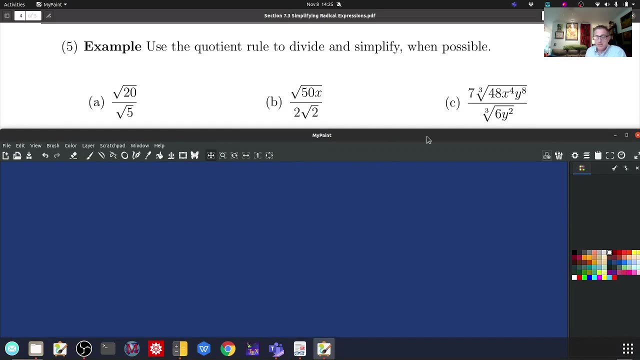 Maybe it's a Mandalorian effect, or whatever Mandela effect- I don't know what it's called. So now we're going to be using the quotient rule. So basically, it's kind of like in music: I've introduced a theme which is a rule, in this case, 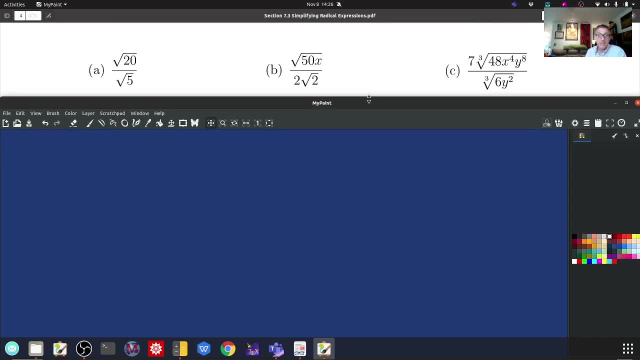 And we're playing variations on that theme or themes. So what problem is this one? This is 4.. So this is 5a, So the square root of 20 divided by the square root of 5.. So we're going to do this. 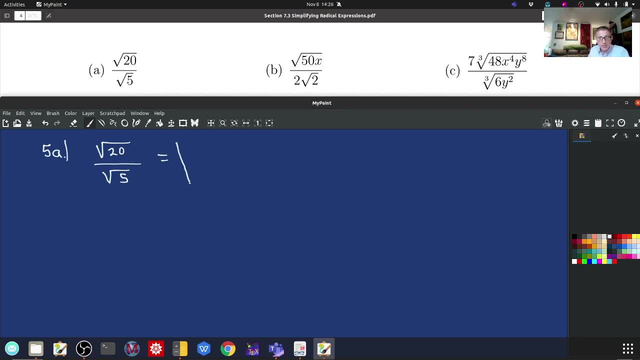 So we're going to do the other direction. This is equal to the square root of 20 divided by 5.. And you should always go this way if the radicand in the numerator is divisible evenly by the radicand in the denominator. 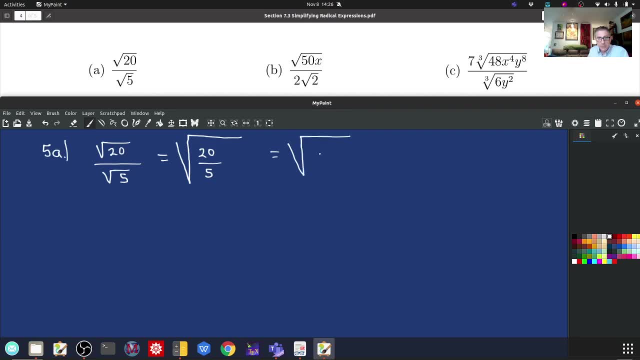 So that's equal to the square root of 4.. And you all know that one That's equal to 2.. So the square root of 50 divided by 2 and the square root of 2.. So you say what's going on here? 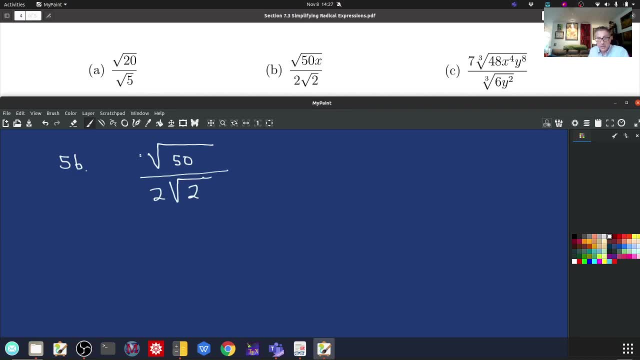 There is a little bit of something going on here, So that's the same thing as 1 half 1 half times the square root of 50 divided by the square root of 2.. Well, that's equal to 1 half times the square root of 50 divided by 2.. 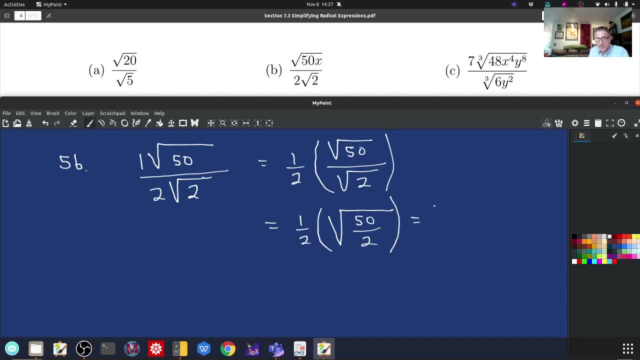 Do you see how this is going to work out? Well, that's equal to 1 half times the square root of 50 divided by 2.. Well, that's equal to 1 half times the square root of 20.. Put that in the numerator. 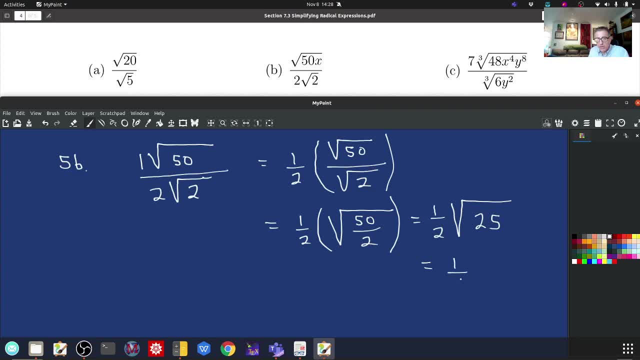 In the numerator procedure And the denominator p n emphasize 1 half times 5.. And p? n single. But up here in the numerator it says it has just square root of 25.. It's the square root of 25, which is equal to 1 half times 5.. 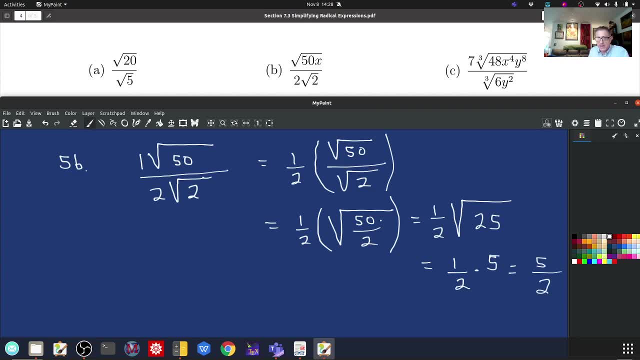 1 half times 5.. Which is equal to 1 half times 5.. 1 half times 5.. Which is equal to five halves. And now I look up at the problem and I see I forgot to copy down and value of x. So I'm just going to go ahead and put it in and that's going to. 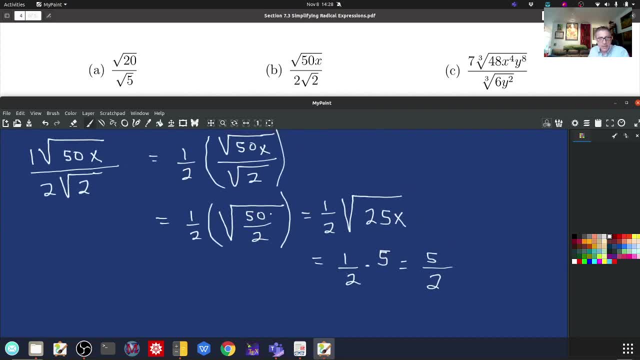 require a slight modification right here. So let me erase. sorry, I apologize. See, if I can't get my eraser to be bigger, We'll start right here. I'll fix it, starting right there. So this is again 1 half. it's a little bit thicker there 1 half times. here I go. 1 half times here I go. So I'm just going to go ahead and put it in and that's going to be 1 half times here I go. So this is again 1 half. it's a little bit thicker there. 1 half times here I go. 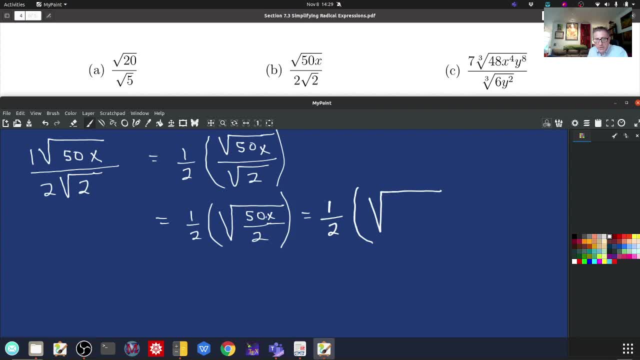 The square root of 50 divided by 2, 25x. Well, that's equal to 1 half times the square root of 5 squared times x. So I can bring: since 2 is divisible by the index, that's equal to 1 half times 5, the x has to remain. 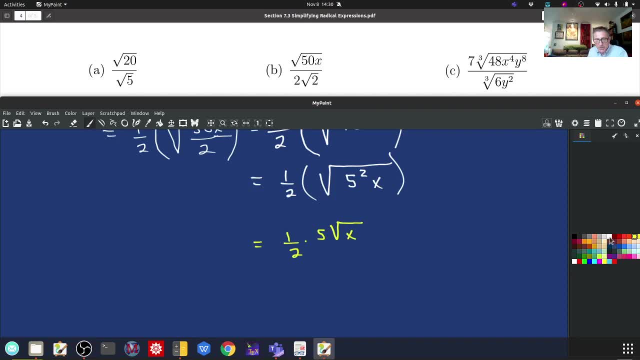 underneath the radical. So another way of writing. that is 5 times the square root of x divided by 2.. Sorry about that, I copied it down wrong. So here's a doozy, or so it seems at first. I'm going to suggest it's not going to be near as bad as it looks. So this is example 5c. 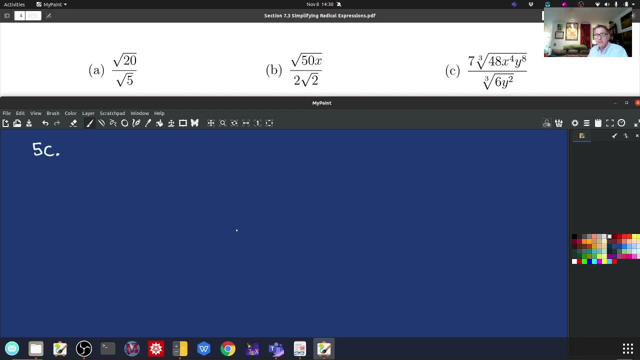 So I'm going to challenge you right now to see what you can do with number 7.. Just kind of look at it. You'll notice that the index is going to be a little bit thicker. So I'm going to challenge you right now to see what you can do with number 7.. Just kind of look at it. 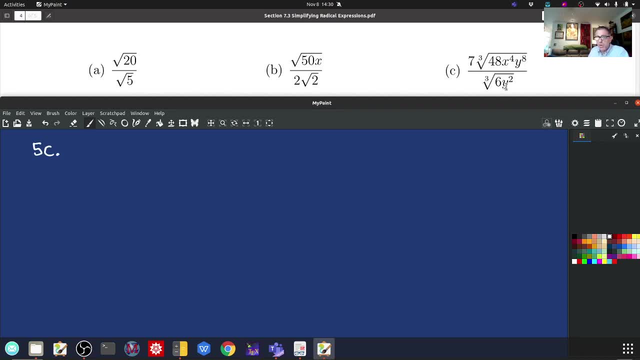 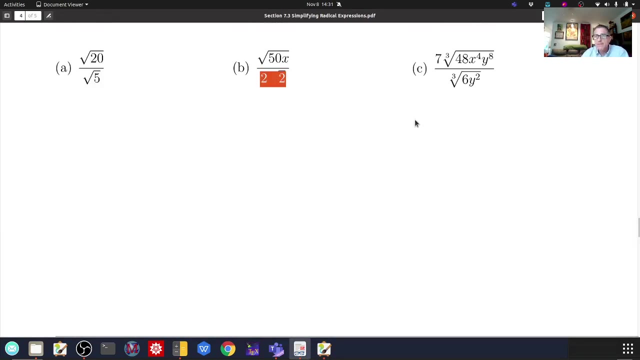 The index is 3.. Now y on the denominator. let's see what you can do there. So you're going to use the quotient rule. Since the indices are the same, you can use the quotient rule. Come back here. So let's just do it. I mean you can pause and do it on your own. 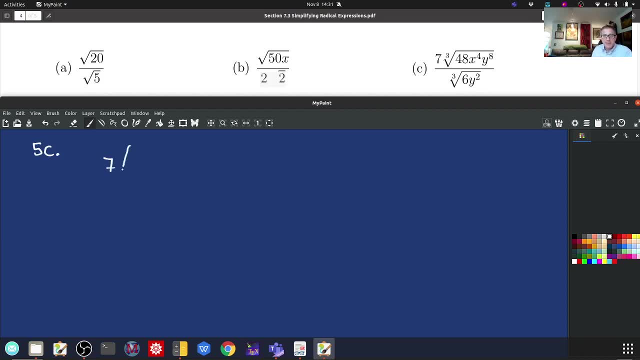 So this is 7 times the cube root of x squared. So this is 7 times the cube root of x squared. So this is 7 times the cube root of x squared. So this is 7 times the cube root of 48x to the 4th, y to the 8th, over the cube root of 6y squared. 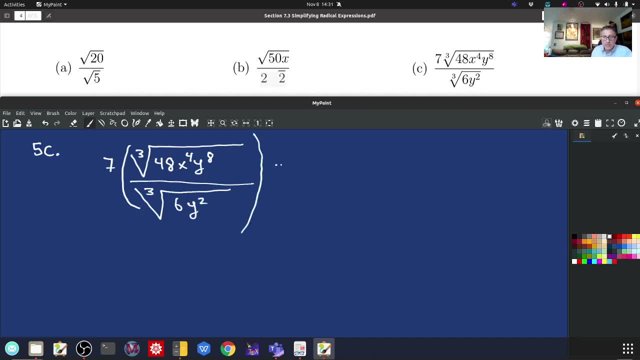 So let's just literally use my, So let's just literally use my index rule. first Let me 7.. That's one big, huge index thingy. It's the index. It's one huge radical And the index is 3.. 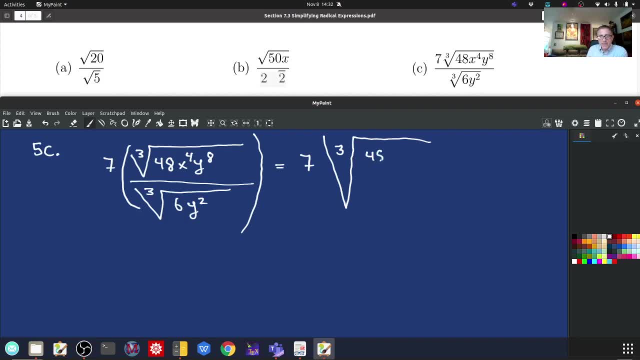 So that's going to be equal to 48x to the 4th y to the 8th divided by 6y. So that's going to be equal to 48x to the 4th y to the 8th, over the cube root of 6y squared. 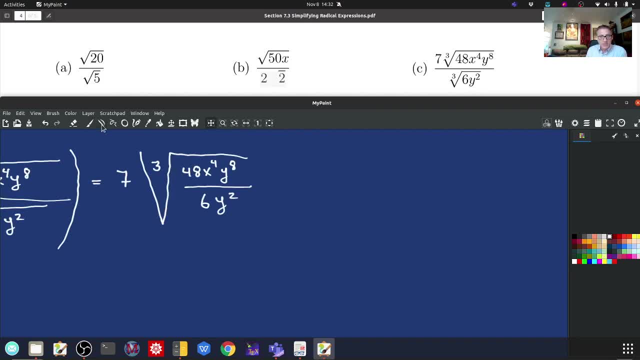 So let's go ahead and simplify this out. I'm hoping you're seeing what I'm seeing. It's going to be far easier. 48 divided by 6 is 8.. x to the 4th stays to the same. x to the 4th stays to the same. 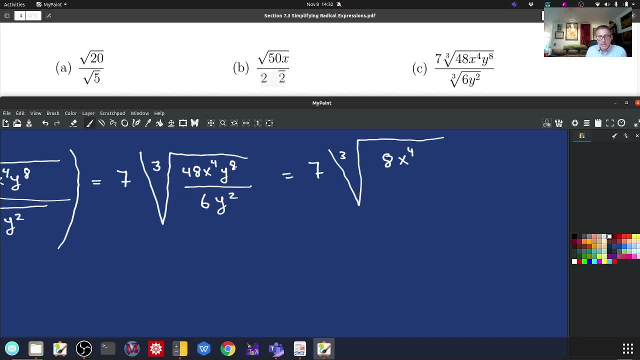 1 to the 4th stays to the same. 1 to the 4th stays to the same. y to the 8th. divided by y squared is y to the 6th. Now recall that 8 is equal to 2 to the 3rd. 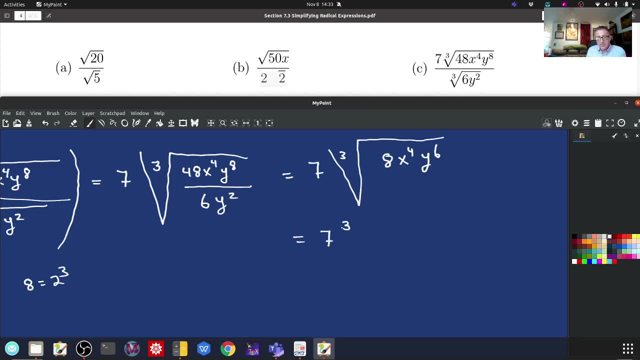 So I have 7 times the cube root. I'm going to write 8 as 2 to the 3rd. I'm going to write x to the 4th as 2 to the 4th- 9 times the 3rd. 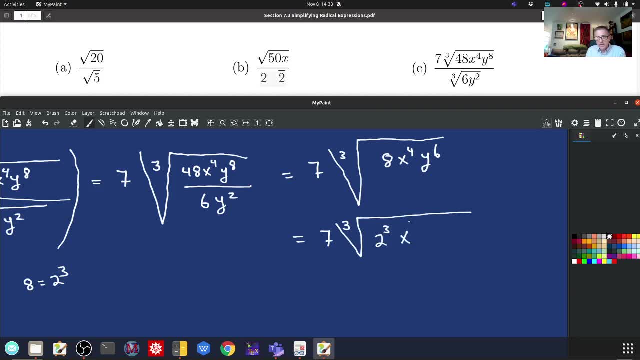 9 times the cube root of 22 to the 3rd, 7 times the cube root of 22 to the 3rd, coming from the 8.. to the fourth is x to the third times one, I'm sorry, x to the first. There we go, And I know I. 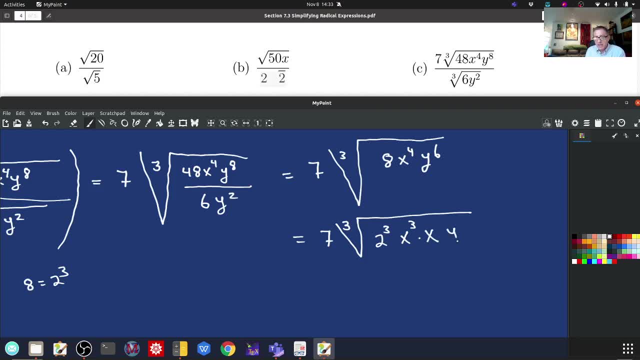 can do that, because four is greater than three, And y to the sixth I don't have to do anything to, because six is evenly divisible by three. Now I'm almost ready. I'm going to bring some stuff out, So that requires me to scoot this seven over, And each thing that I bring out, seven is going to. 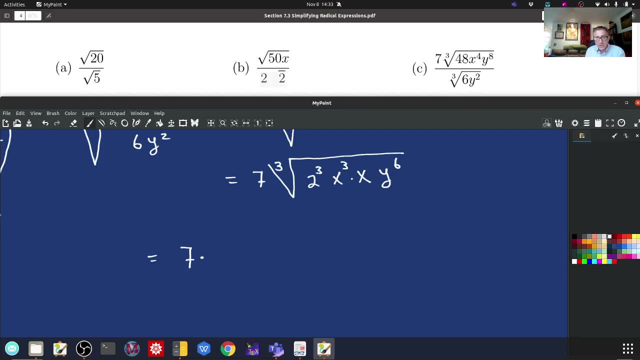 be multiplied by it. So two to the third divided by three is two to the first. Now I can bring out x to the third, x to the third divided by three is x, y to the sixth. Six is divided by three is y squared. And what did I? 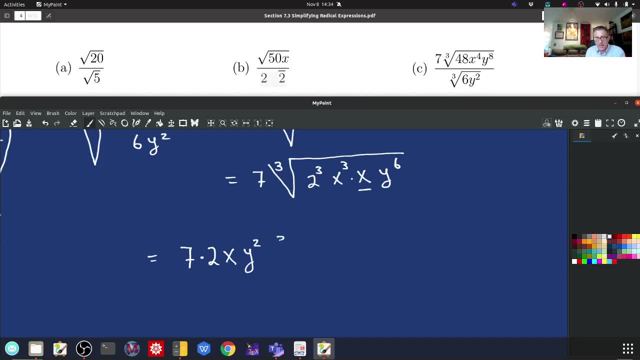 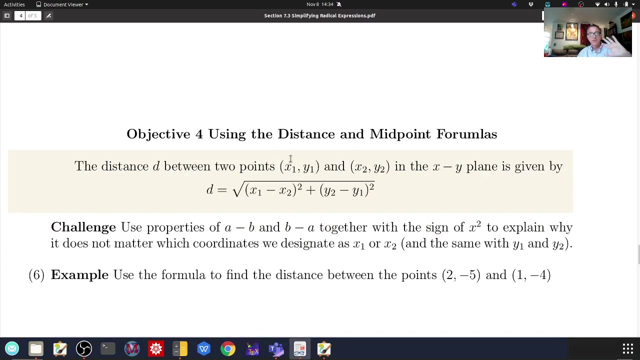 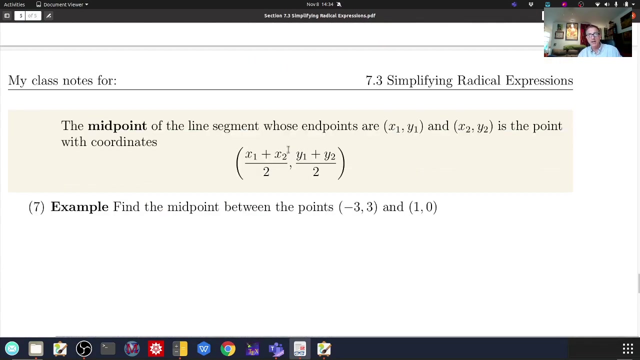 Well, it has to remain just this one factor of x. So it's the cube root of x. So seven times two is 14.. x, y squared times the cube root of x. Okay, that's it. We don't do the distance and midpoint formulas. That is not part of what we do in intermediate algebra. You'll 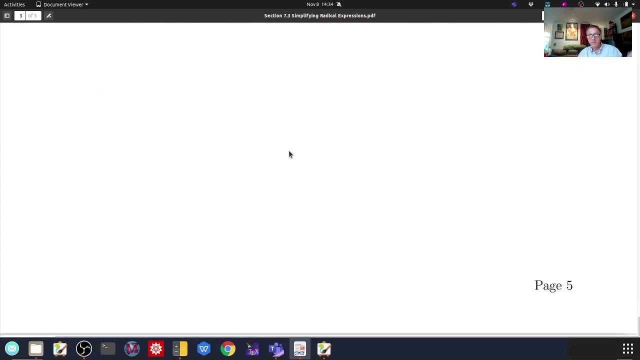 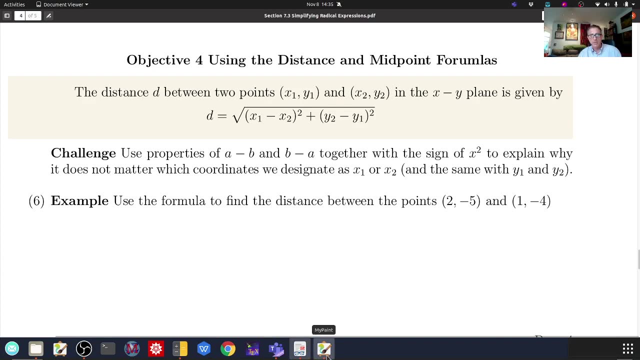 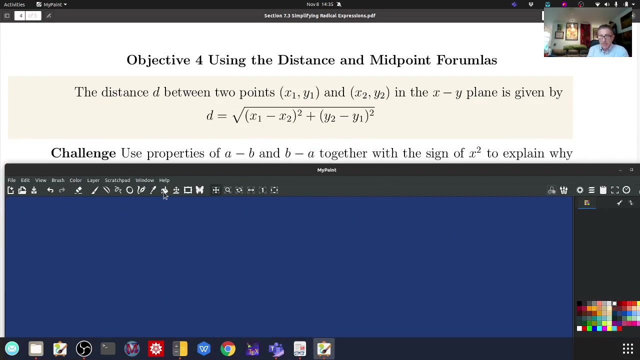 do that in college algebra. So from here on down, as far as the notes go, you can absolutely ignore them, And I'll write a little note here just in case you're going through fast forward. I'm just going to say: ignore midpoint, And I've changed your homework to not include midpoint or distance. 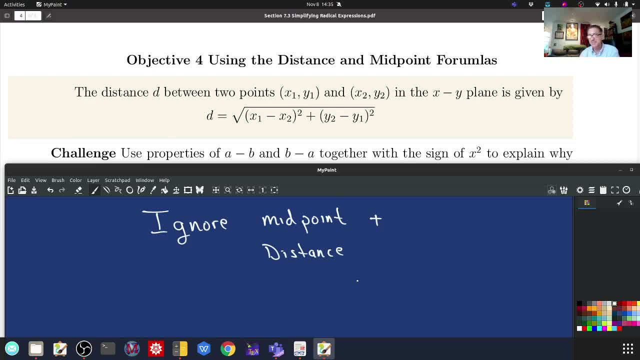 problems. Okay, that's it for 7.3..